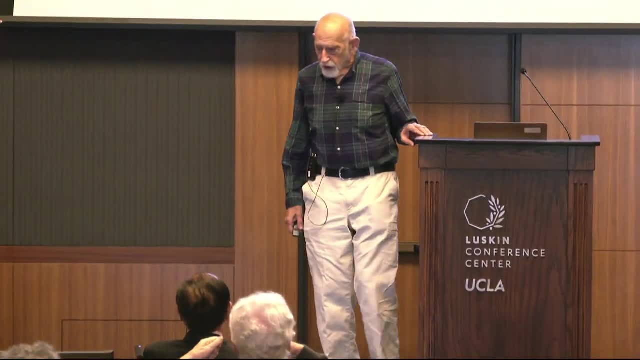 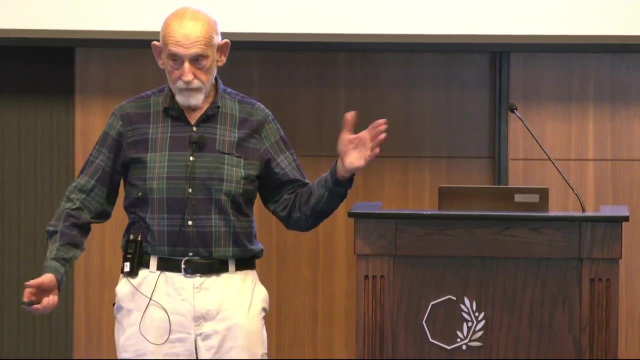 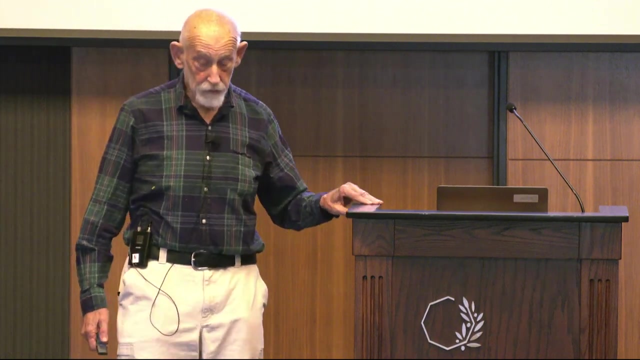 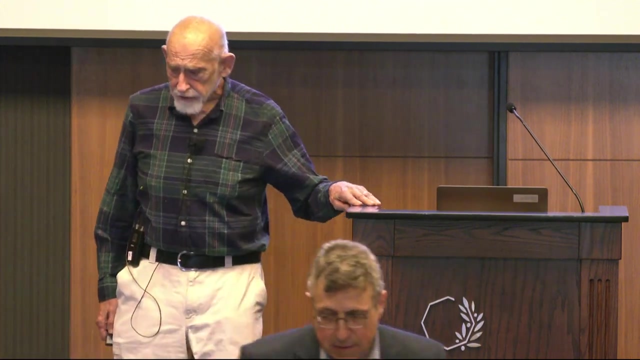 Thank you, Thuy. My talk today is going to be unabashedly about myself and my relationship to QCD. Now, the last paper I wrote on QCD was 43 years ago. It's true, It was not about confinement, It was about de-confinement of high temperatures. So I've been away. 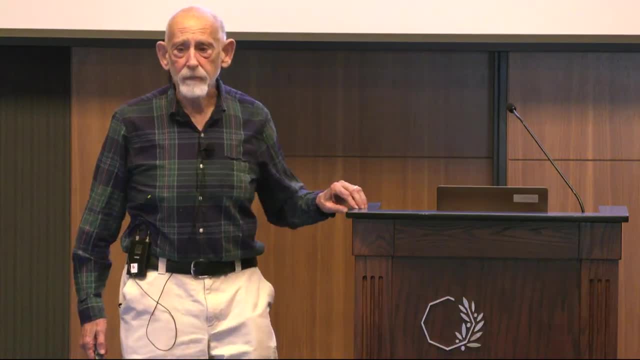 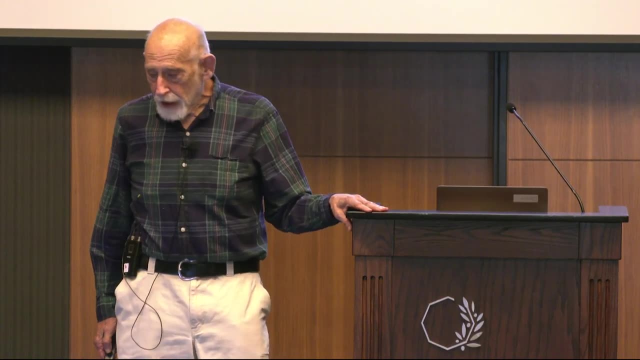 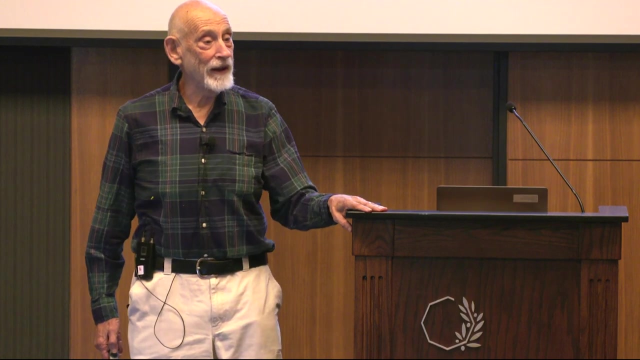 from it for a long time. I feel a bit like Odysseus coming back to Ithaca after the Trojan Wars- Well, I suppose after the Black Hole Wars- And it feels good. I'm really happy to be here. I'm enjoying thinking again about what was my first love in physics: Hadron's. 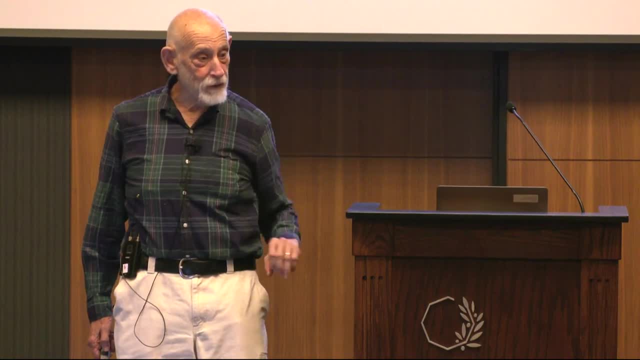 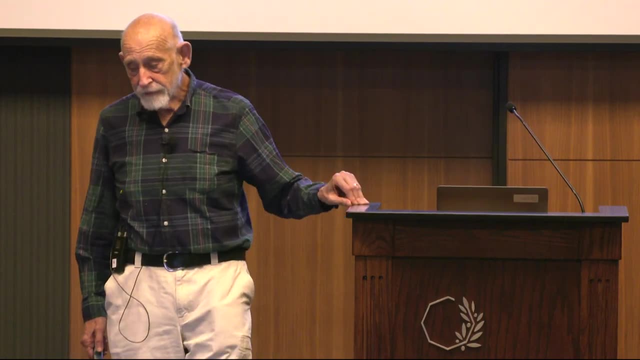 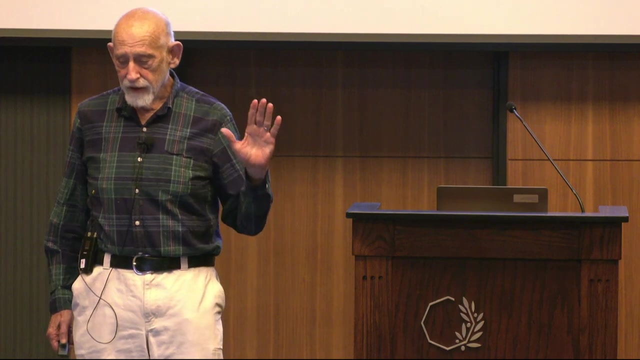 QCD, And so happy birthday, QCD. Okay, We're going to have a little break, Thank you. We're going to talk about the confinement mechanism. The first thing to mention is that the confinement mechanism is not asymptotic freedom. Asymptotic freedom plays a tremendously. 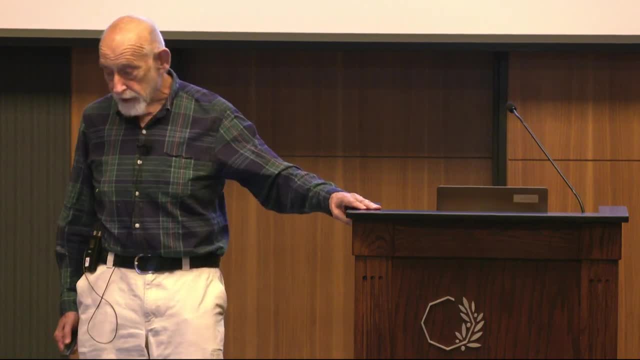 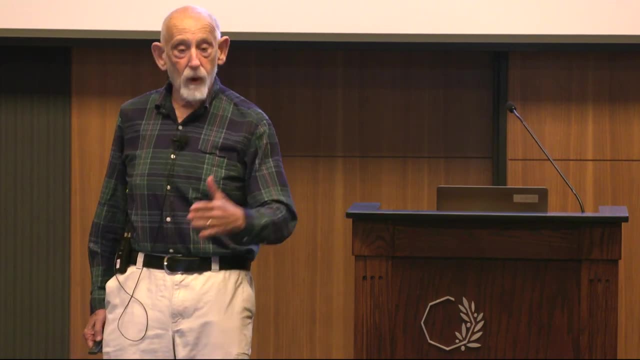 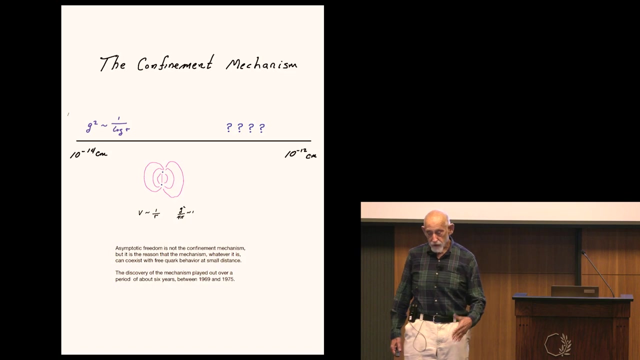 large role in confinement. What asymptotic freedom tells us is how to continue away from intermediate coupling, let's say, at a few times 10 to the minus 13 centimeters, how to continue to very small distances. It leaves open the question of what the physical mechanism 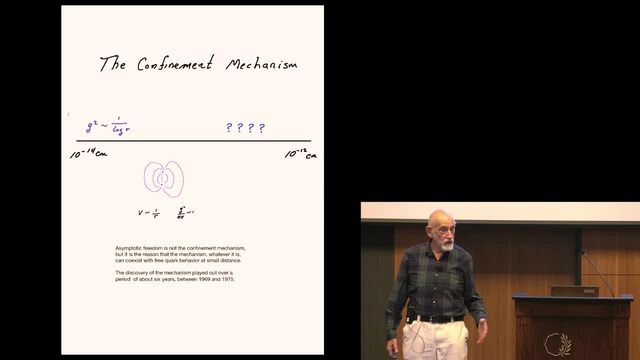 at longer distances, which controls all sorts of things such as confinement, nuclear physics and so forth, And that's what we're going to talk about today, the other end of the spectrum of energies, the infrared. Now, as I said, asentonic freedom is not the confinement. 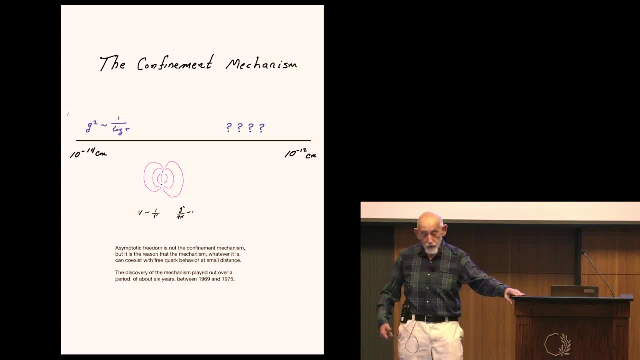 mechanism. But it's the reason we think, you know, confinement requires these things, The reason that the confinement mechanism, whatever it is, can coexist with freakwalk behavior at small distances. The discovery of that mechanism played out over a period, in my view, of about six years. 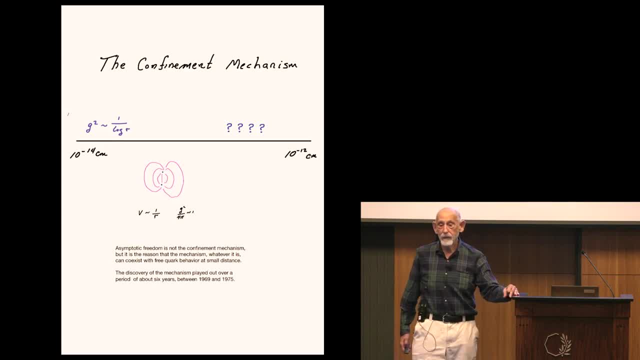 between 1969, which is probably the only person- I don't know how many people here- were physicists in 1969, I know that guy was, but I am older than David, so my memory is a little longer. Anyway, that's what we're going to talk about. 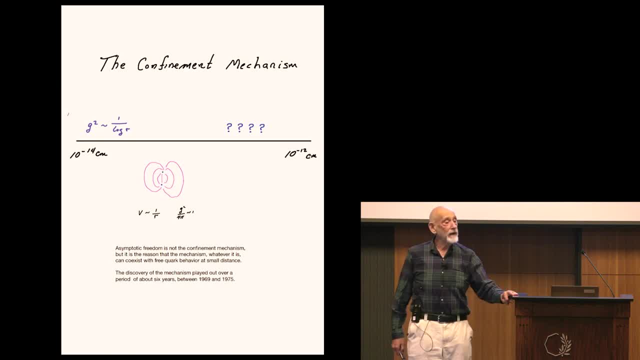 But I'm going to go back a little further, actually, to the time that I first met David, which was 1965. At that time there were basically two schools of thought about hadrons. I would call them the Berkeley School and the Caltech School. 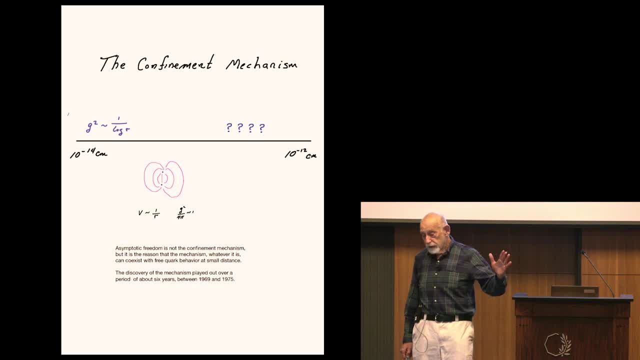 In the Berkeley School, quantum field theory had been completely rejected as a way of thinking about hadrons. The right way, at least according According to the Berkeley School- was the black box picture, the S matrix. That's all there is and that's all there will ever be. 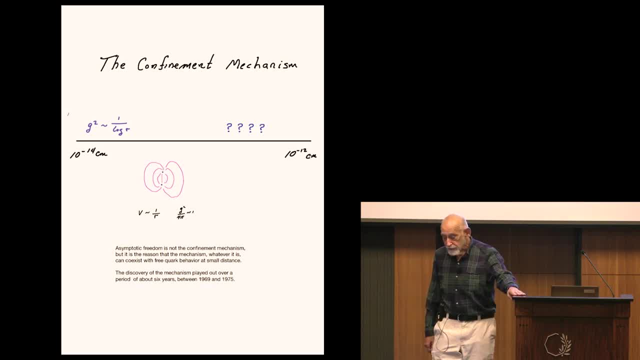 In principle, no experiment can open the black box. Hadronic physics takes place on scales which are much too small and too fast to resolve. Unitarity, Lorentz, invariance and analyticity were the mathematical rules that, if you use them repeatedly, you could bootstrap your way to the S matrix. 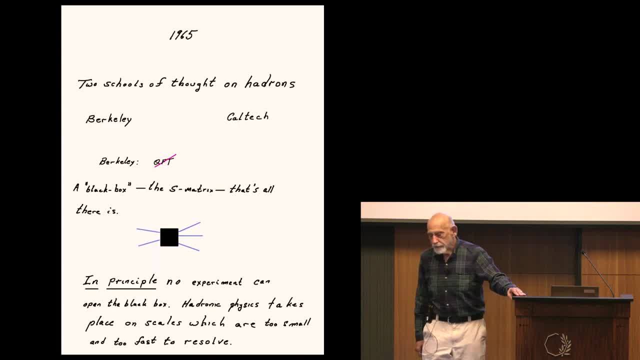 Thank you. It was a bit of a mashup of ideas, some good, some not so good. One of the good ones was the two Fauci plot regi trajectories for real particles, For reasons I was never able to comprehend, since I don't believe at that time there were. 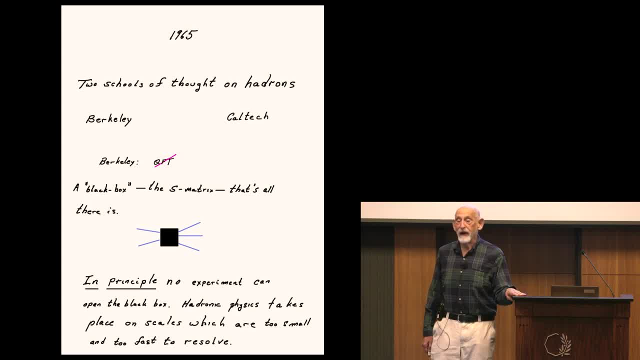 more than two particles on a regi trajectory, if that many, For reasons that are hard to understand. maybe it's a theorem. there's a theorem that says through any two points you can draw a straight line. You're supposed to laugh at that. 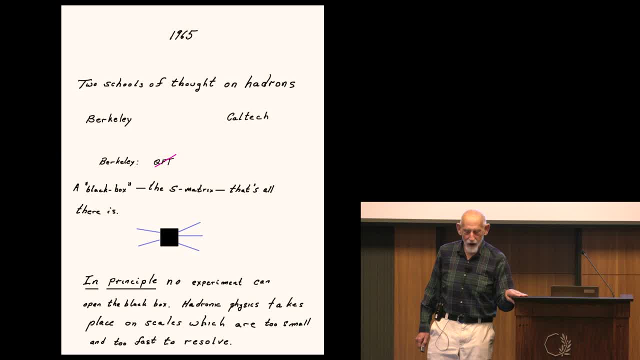 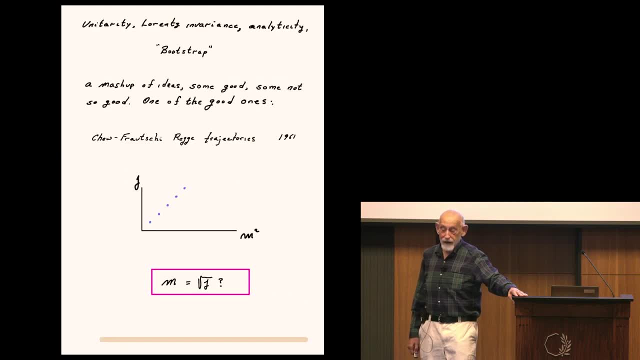 Anyway, Chu and Fauci drew a straight line and said: regi, trajectories are straight lines. That meant that the mass squared and the angular momentum of particles were linearly related to each other. Notice it's mass squared, or mass, is proportional to the square root of the angular momentum. 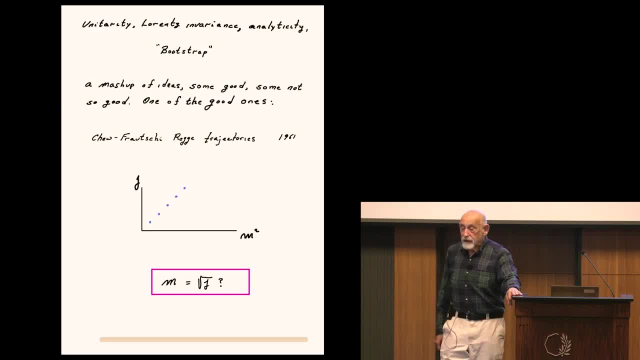 square root of an integer. Now, the Caltech view focused on flavor symmetries. Okay, SU3 cross SU3, left cross right. no color, just flavor symmetries. approximate conservation laws and the coupling of hadrons to photons and leptons. 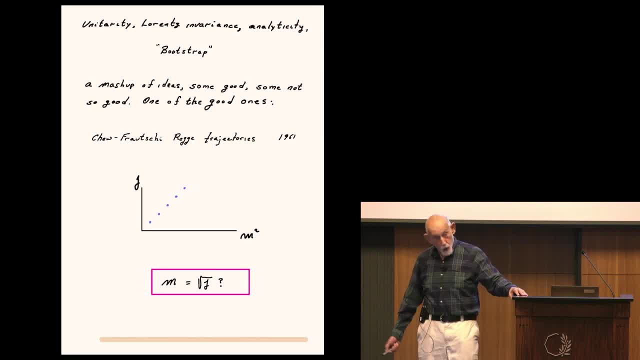 The currents of the weak and electromagnetic interactions, according to the Caltech school, behaved as though hadrons were collections of freak walks. Gell-Mann made the statement, which is a bit trite. he said that nature reads books on free-feel theory. 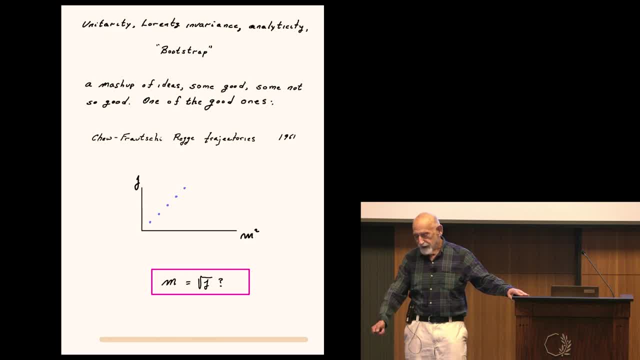 One of the less interesting things I thought he ever had to say, but he said it. My own view at the time, and somewhat later, was that we should open the black box. We can stretch things out, slow them down in order to observe their internal motions. 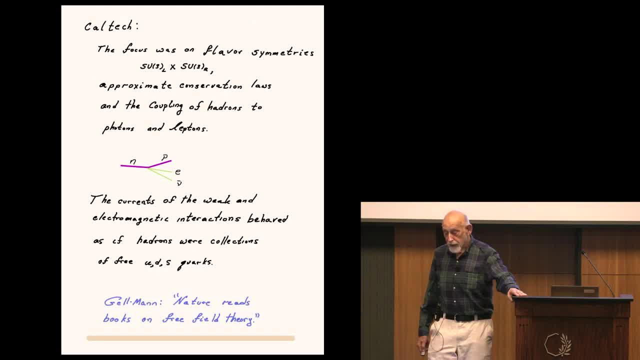 And what's the trick for that? What I called at the time the infinite momentum frame. The infinite momentum frame is just a frame where everything is moving very fast. It had been studied by Weinberg in 1968.. It was a very interesting experiment. 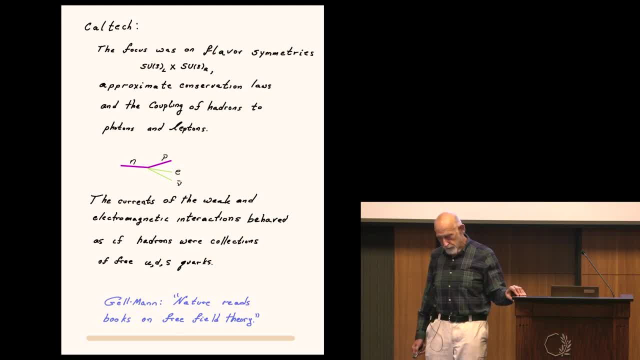 It was a very interesting experiment. In 1966, he studied Feynman diagrams in the infinite momentum frame. I also studied it in 1968, and in particular studied about how to do quantum mechanics in the infinite momentum frame And in particular, is there a Hamiltonian? 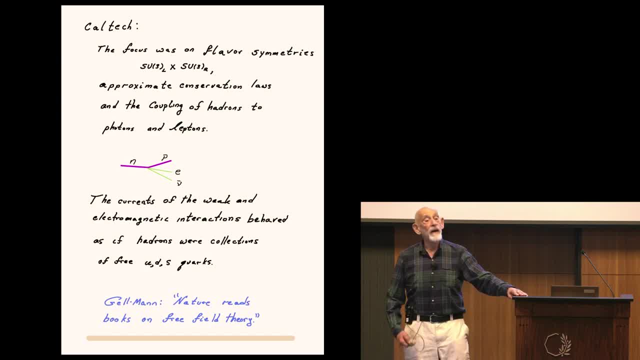 Is there a space of states And what are the symmetries? One of the discoveries was that the symmetries included a Galilean subgroup which made infinite momentum physics look very, very much like Galilean non-relativism. 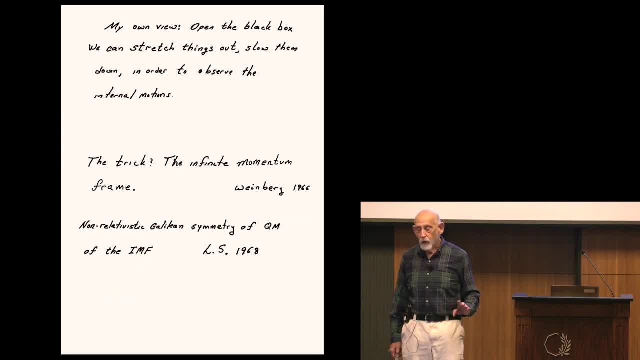 And that's the reason why we have a lot of physics. But for our purposes here, the important thing to know is that when something moves fast, it moves very slow. If it's moving fast past you, its internal motions are slowed down. 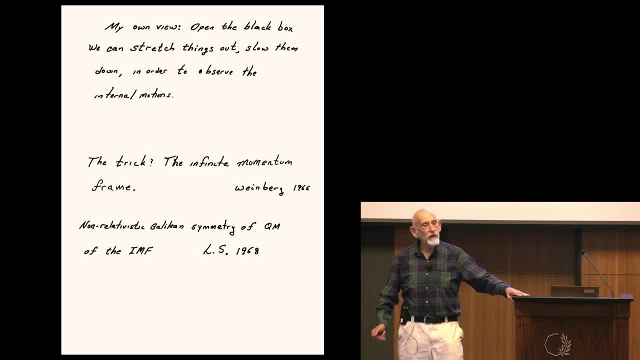 So the idea which I published as a paper said: consider some hydronic system in a frame in which it's moving very, very fast or close to the speed of light, And now imagine putting something in the way so it gets excited. 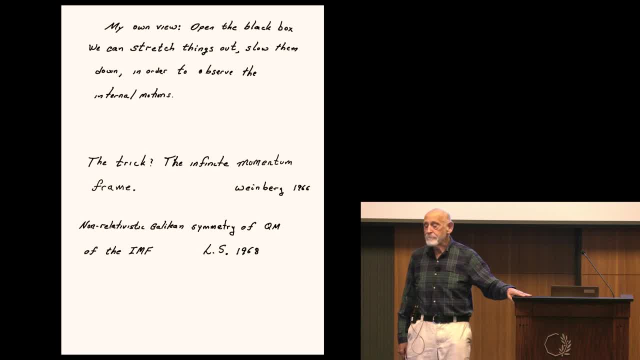 So the thing passing through it gets excited, It starts vibrating or whatever, And now stationed downstream, at different distances, detectors. What you have then is this stretched out situation where the internal motions are so slowed down that you can see them evolving by putting your detectors at different distances downstream. 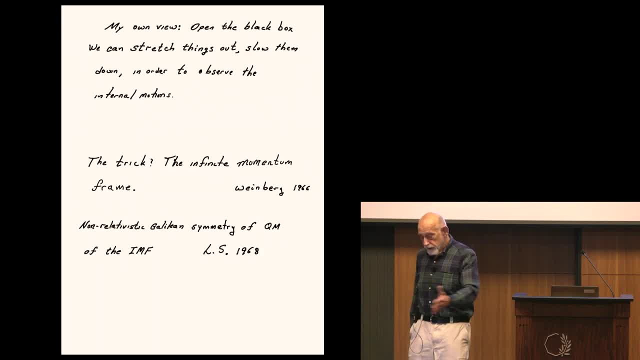 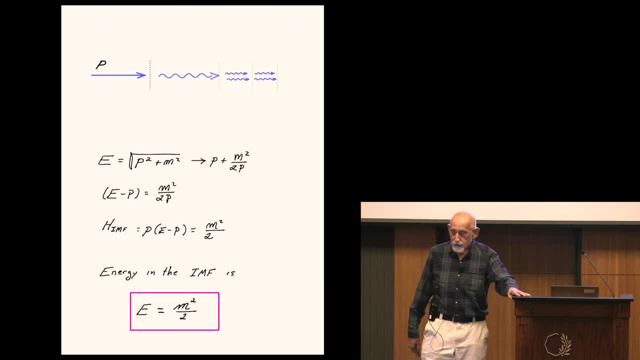 There's a Hamiltonian that governs this internal motion. You can work it out. I won't work it out for you. Most of you probably know it. What it says is the energy. the relevant energy in the infinite momentum frame is the square. 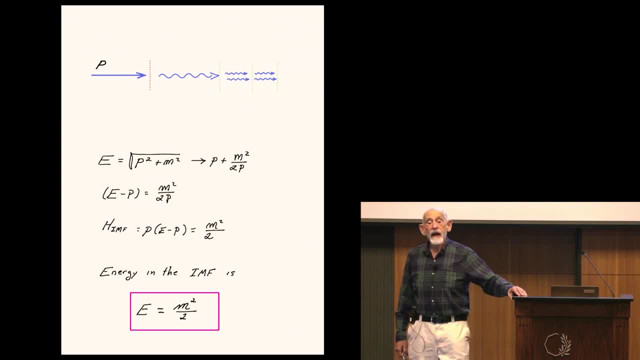 of the mass. not E equals mc squared, but just E equals m squared over 2, where m means, if you like, the mass, but really just the center of mass energy. OK, Now let's. that was interesting. 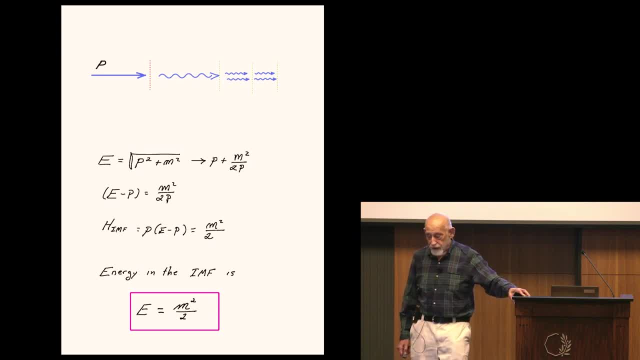 Why was that particularly interesting? Well, it was interesting, Why, Let's go back, Let's go back. E equals m squared over 2.. And the true Frouchi plot- whoops, sorry, The true Frouchi plot- said that m squared is proportional to j. 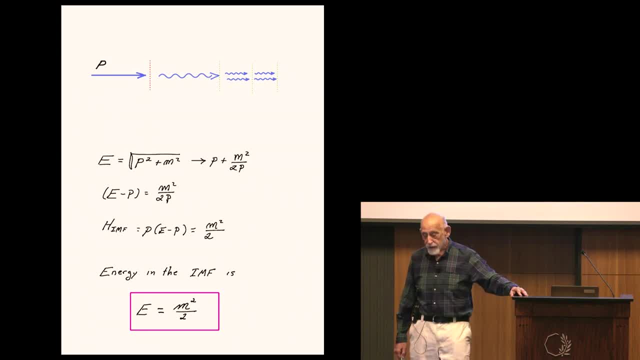 What this said is: the energy in the infinite momentum frame is j, which is integer spaced. It meant to me that hadrons are harmonic oscillators. Let's go back to the S matrix for a minute. By 1968, Veneziano had conducted an experiment. 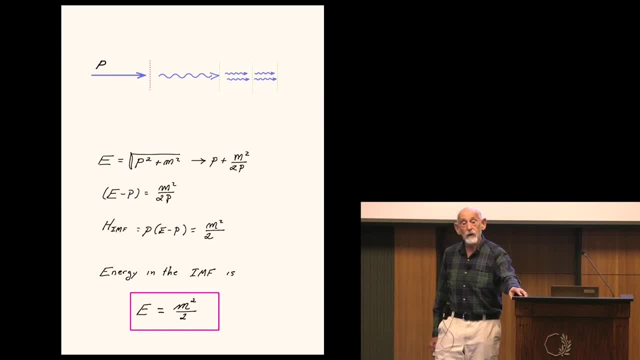 Veneziano had constructed a fantastic solution to the bootstrap equation. I don't know if it was to the bootstrap. You can tell me Were you thinking about bootstrap? I have no idea. But you just magically, magically and brilliantly put together a formula. 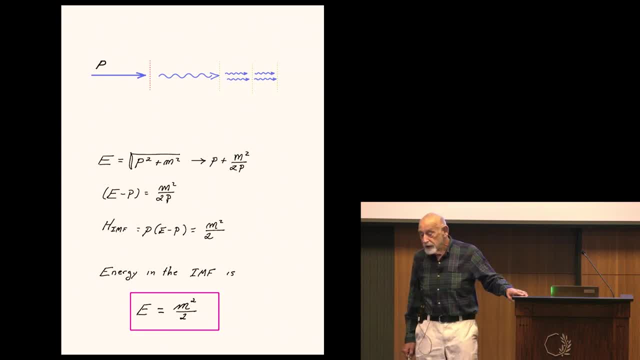 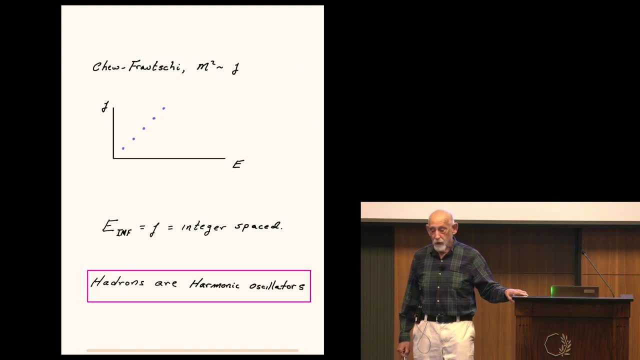 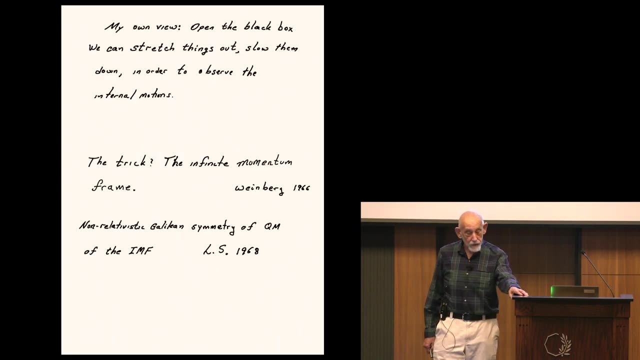 You probably all recognize it: It's the Veneziano amplitude, And it can be written as an integral or a product of gamma functions. This was an earthquake to me When I saw it. not only did it have linear register trajectories, but it had an infinite. 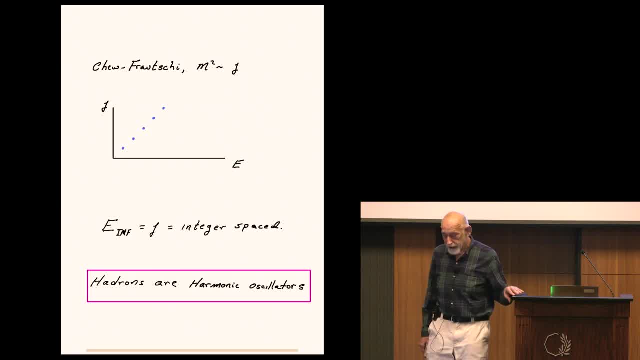 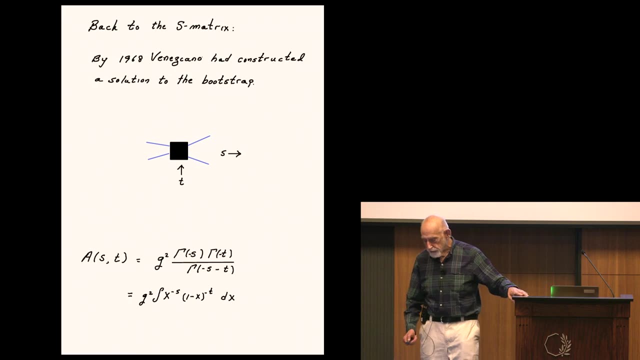 sequence of so-called daughter trajectories, which we'll come back to if we have time. But it was also exactly the spectrum of a two- or three-dimensional oscillator. Oscillators: when they rotate, they can vibrate. They have exactly this kind of daughter spectrum. 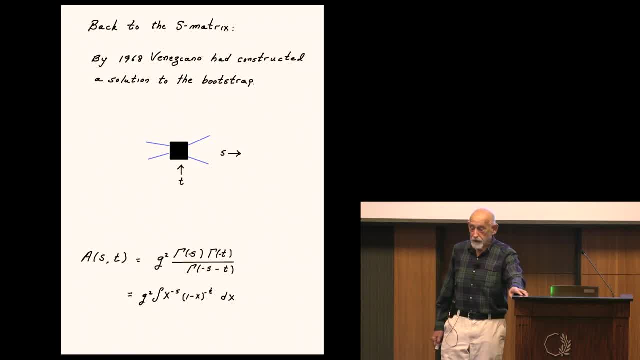 And so that led me first of all to start thinking about this harmonic equation. I was thinking about this harmonic oscillator analogy for hadrons. I don't know exactly what was in Nambu's mind, but I suspect it was very similar. 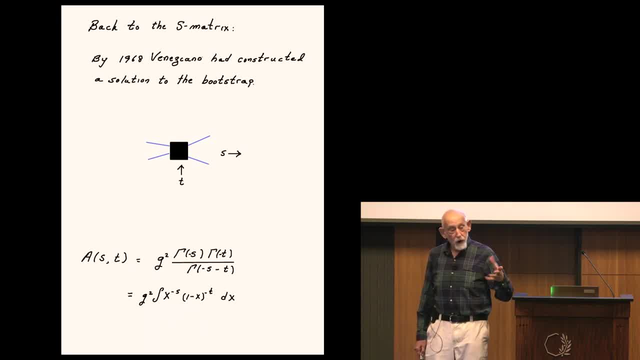 Start with a harmonic oscillator, a spring, if you like, with a quark at one end or quarks at both ends, if you like, and scatter a photon off it or scatter whatever you like off it, And you can calculate scattering amplitudes for this kind of thing. 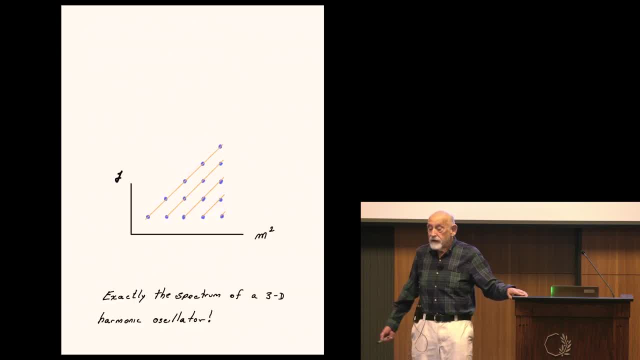 You absorb a photon, You re-emit the photon And it's an answer which looks vaguely like the Veneziano amplitude: Instead of 1 minus x to the minus t, it was e to the minus x to the minus t. Well, when I saw that, when I realized that, I immediately started to think: how do you? 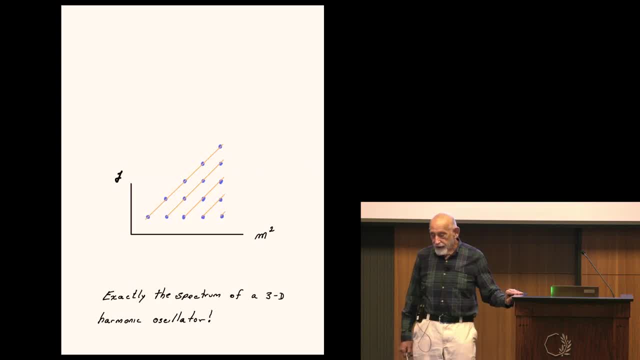 go from e to the minus x to 1 minus x, And the answer is that 1 minus x to the minus t is an infinite product: e to the x to the minus t. You can work this out And it's a. it's an easy one, It's a high school algebra thing. e to the xt to the x squared T. 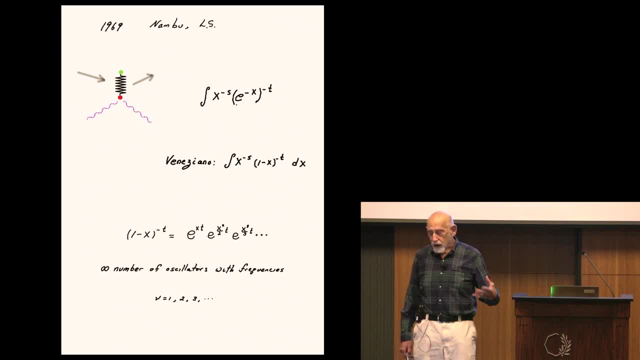 And what it meant is that the Venetiano amplitude Corresponded not to a spring, but some kind of infinite set of normal modes with frequencies 1, 2, 3 and so forth. In other words, it was a string. Spring theory had become string theory. 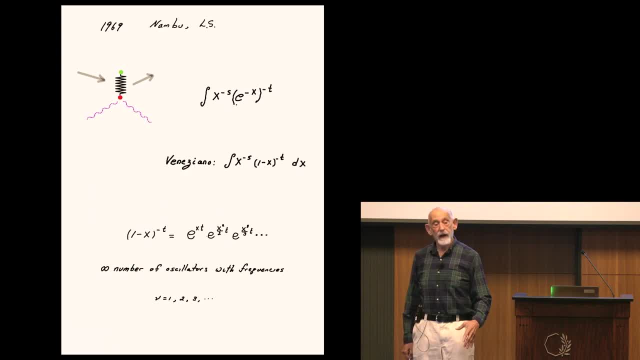 Once you realize that a mezzan, let's say, is a string, you immediately start drawing space-time diagrams in which the world line of a particle is replaced by a two-dimensional sheet with quarks at the boundaries. The world line becomes a world sheet. I think I coined that term, but maybe somebody else wants to take credit for it. I'm not sure. 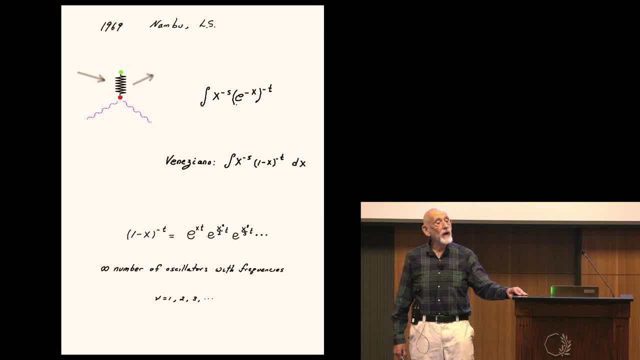 Here's another picture of a world sheet- You probably recognize it- with quarks running around the boundaries. this idea of a diagram like this- not in string theory, but just a Diagram with quarks having this kind of configuration- had already been used phenomenologically by Chan and Peyton, Harari and Rosner and was known to be a reasonably successful description of. 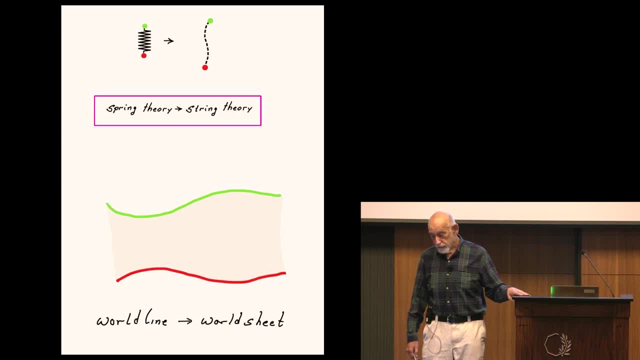 the Quantum number dependence of scattering amplitudes. now there's somebody else I should mention here, and that was Holger Becker Nielsen. Holger had a similar theory, or a Kind of string theory. He didn't call it a string theory, He called it the conducting disk model. the conducting disk model. 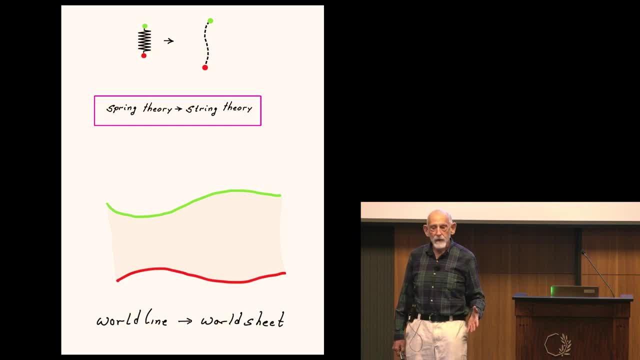 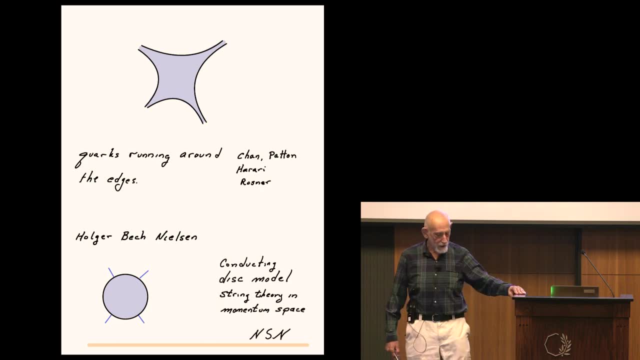 Let's just let me let me just simplify it and say what it corresponded to Was string theory, but not in coordinate space, where you had X's which moved around, but basically in momentum space. if I were to attribute credit to this, to this idea of strings, 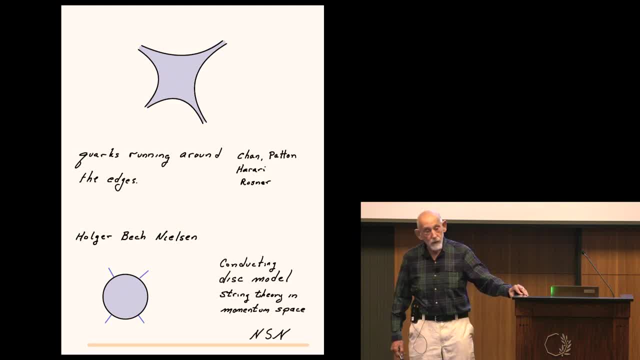 Coming from the Veneziano amplitude. I would attribute it to Nambu myself, Nielsen and I Had a lot of fun talking with Holger about this. I unfortunately never got to talk to the member very much. Anyway, let's come back. The infinite momentum frame, energy, is M squared or M squared over 2 in this harmonic oscillator analogy. 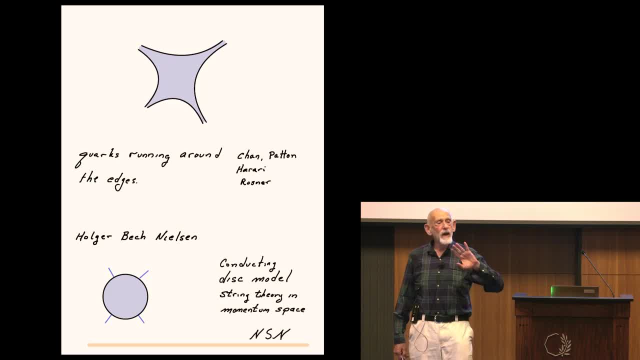 that's equal to some kinetic energy, some potential energy. and You can forget the kinetic energy for this purpose. Trust me, I'm a theoretical physicist, You can trust me. You can forget the kinetic energy for a moment and realize that for a harmonic oscillator, 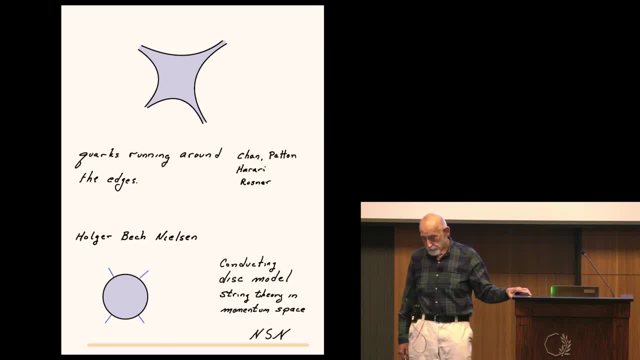 the potential energy has to be proportional to the square of the separation. Well, if you take the square root of both sides, it says the mass or the energy, or in this case, the potential energy must be proportional to the separation in the rest frame. in the rest frame. 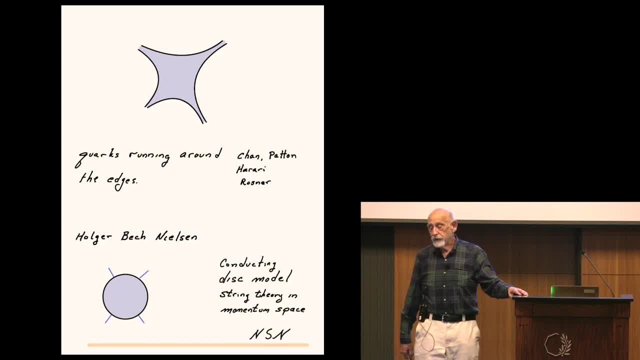 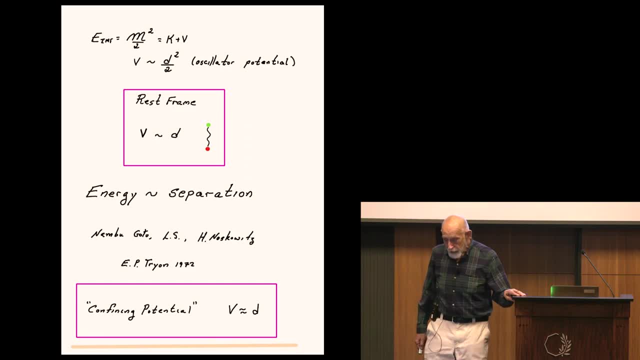 Energy is proportional to the separation. This was the first example, I know, or the first reason that we started thinking about energy proportional to separation. This idea appeared roughly simultaneously in the Nambu Goto paper, a paper of mine, And I also want to point out that there. 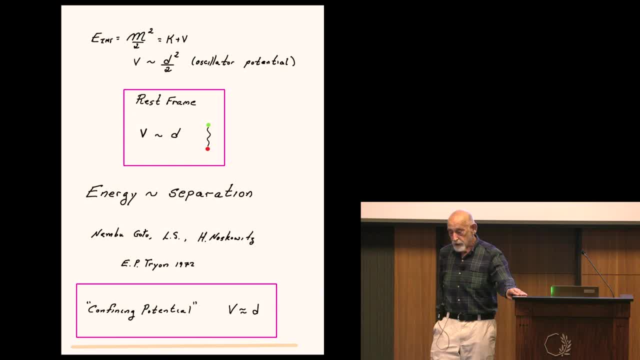 was a graduate student in Tel Aviv University who worked it out by himself. His name was Henri Noskowitz. He was from Belgium. He ultimately left physics- I'm not exactly sure Why- And a version of it appeared in a paper by Ed Tryon. 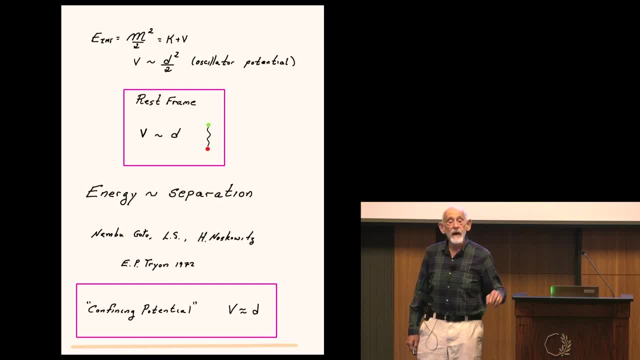 somewhat later, 1972.. The reason I call attention to it is because I think it was a beautiful idea that he had. I recommend that. I'm just going to tell you how to understand the fact that the energy grows linearly with separation. 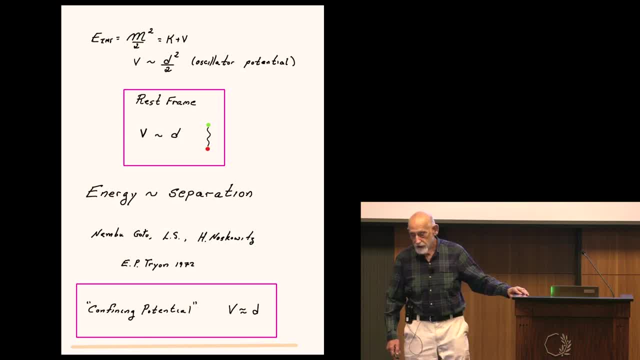 But in any case that was the output of these ideas. It immediately came to mind: is this kind of confinement, linear potentials? is it possible in a genuine quantum field theory? So, sometime around 1972, Aaron Kasher myself, John Kogut. 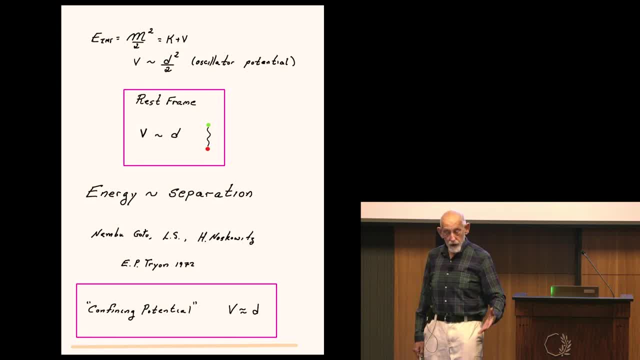 in Tel Aviv began to ask that question: Is there a quantum field theory that can do this? Frankl has already talked about it. Well, first of all, we concluded only in a theory with vector forces. You can read why Scalar forces simply were not. 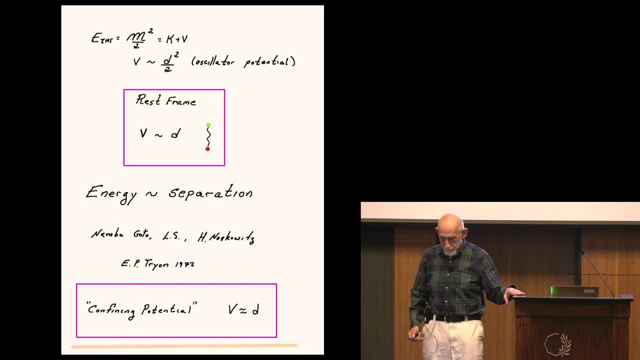 They would not do this. Vector forces might or might not. The simplest example that we could think of to try to work these things out in and see if confinement was at all possible was the Schwinger model, the 1 plus 1 dimensional QED. 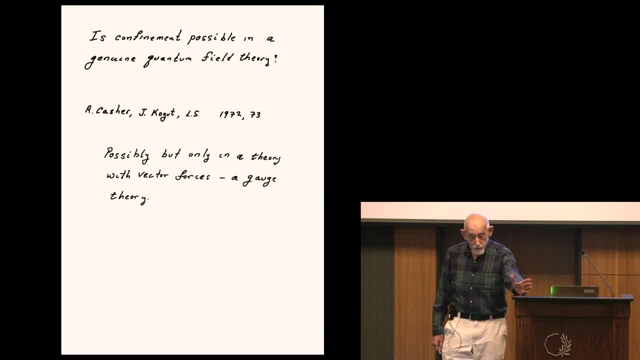 We referred to the charged particles as quarks And, as Frank has already mentioned, confinement of this kind linear potentials is extremely natural. A plus quark and a minus quark will have a line of flux between them. Notice that continuity of Gauss's law, the 1 plus 1. 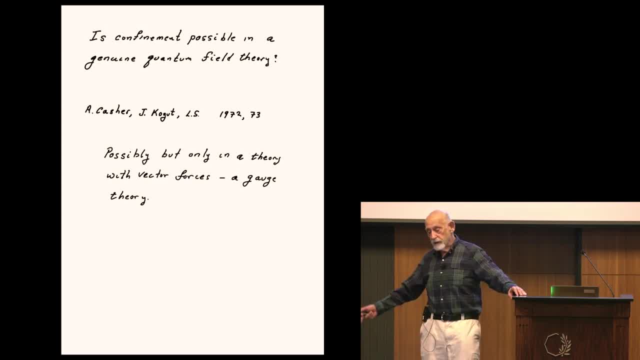 dimension tells us that every charged particle has a line of flux connected to it. The electrostatic energy in that line of flux gives an energy, And that energy is indeed proportional to the distance between the quarks. So electric flux lines in that theory. 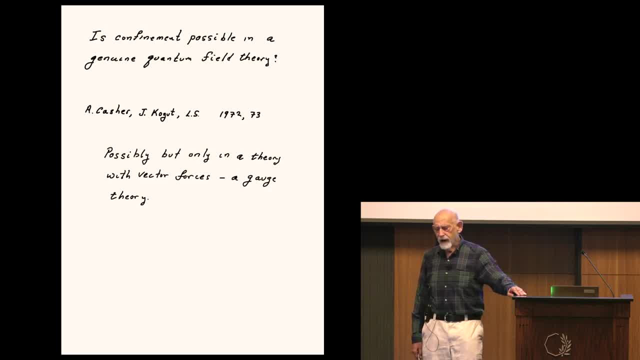 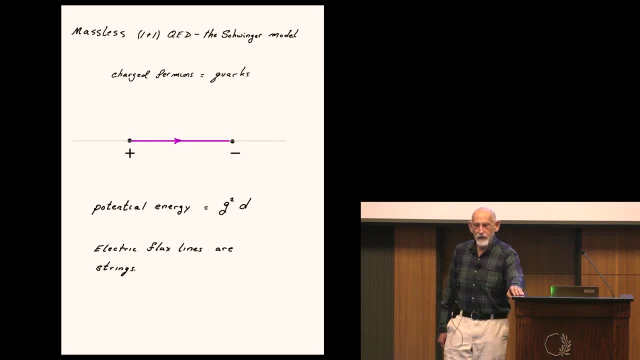 are the analogs of strings. The Schwinger paper I found very difficult to understand, but the model was so easy to solve- It was as Frank pointed out- that I didn't bother trying to read it, just work it out And the solution was simple. 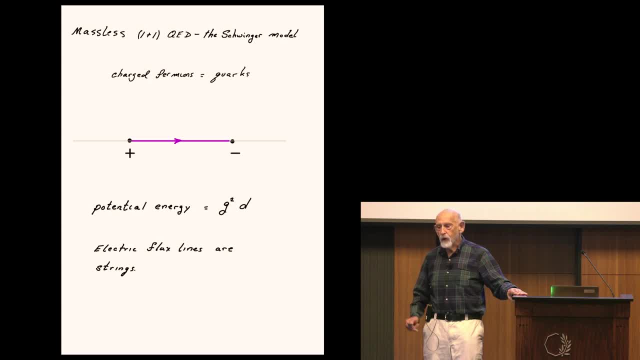 Massive neutral bosons and no charged quarks. It confined. In fact the bosons had properties very similar to hadrons, to mesons, especially in the massive case. John Kogan and I had referred a little bit to the massive case in one paper and Sidney. 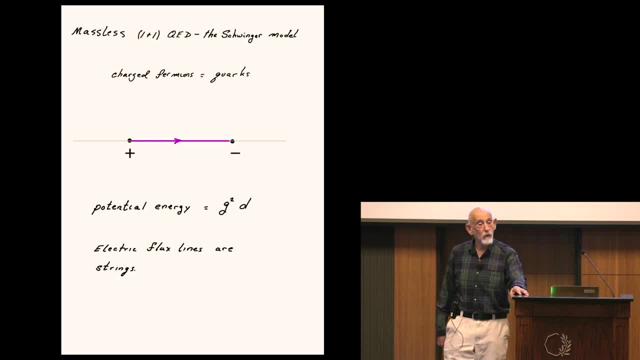 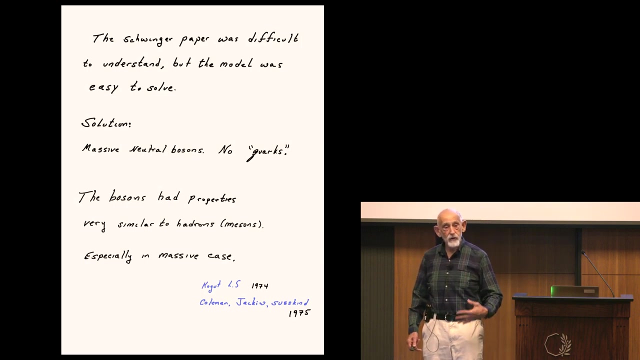 Coleman Jakiv, Roman Jakiv and myself wrote a paper in 1975 about confinement in the massive Schwinger model. It had some properties which are familiar from QCD now. In particular it had an axial current anomaly. It had a potential way to understand the strange U1. 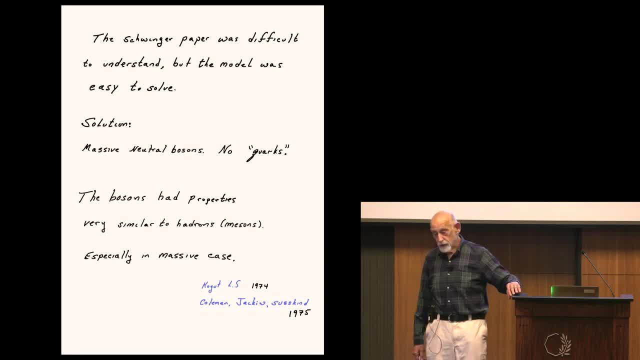 problems that occurred later in QCD or that occurred in particle physics, For example the eta to 3 pi. I vaguely remember what that is: The eta to 3 pi puzzle, the existence of a CP violating C in two dimensions. 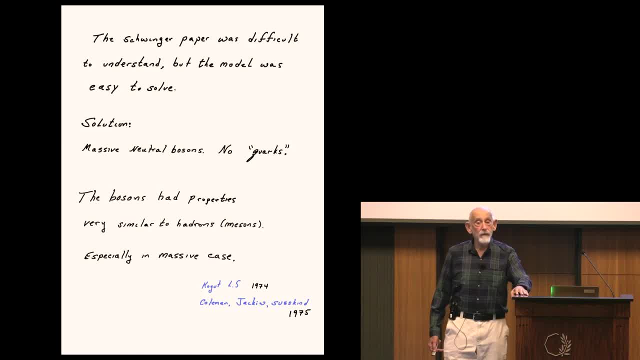 C, violating theta angle. I believe, although I'm not absolutely certain, that this was the first paper that had this idea of a CP violating phase, But I can tell you that it was not due to me and it was not due to Roman. 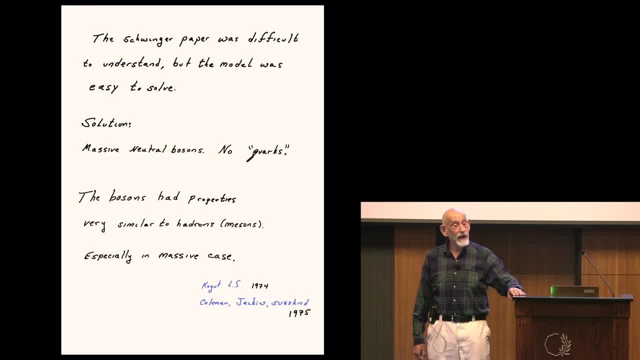 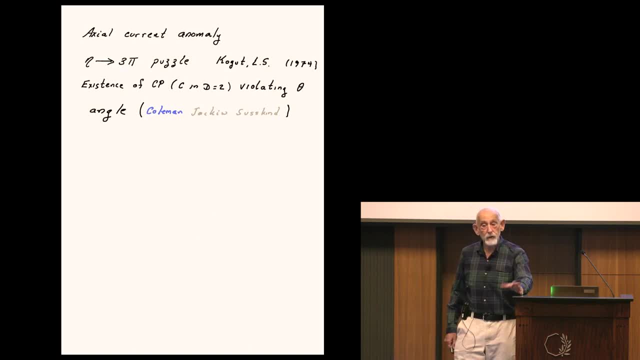 It was strictly due to Sidney, who had been thinking about it for over a year by the time we wrote this paper. So that was the Schwinger model, the role the Schwinger model played in understanding confinement. Later, about a year later, Atoft went further. 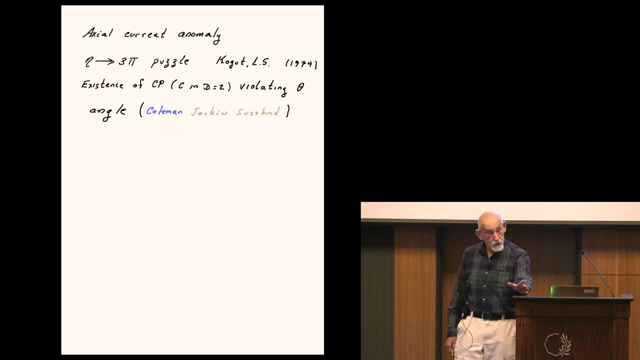 and solved the large end non-abelian Schwinger model using infinite momentum techniques. He found, of course, that quarks are confined. There's a spectrum of color-neutral mesons, The potential energy between them is proportional to the distance And indeed they formed reggae-like trajectories. 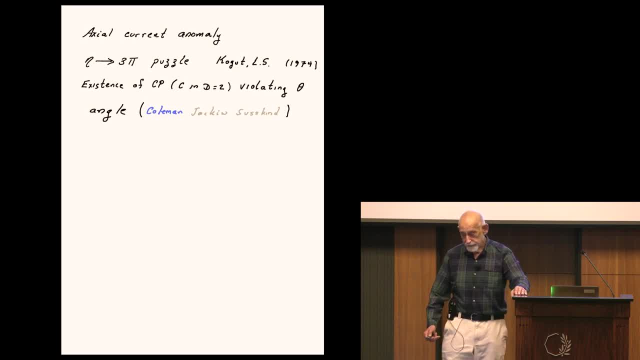 So, yes, a quantum field theory can confine, But can a quantum field theory confine in four dimensions? That was a much harder question To this day. I think it's not a proven mathematical fact, But as we were beginning to think, 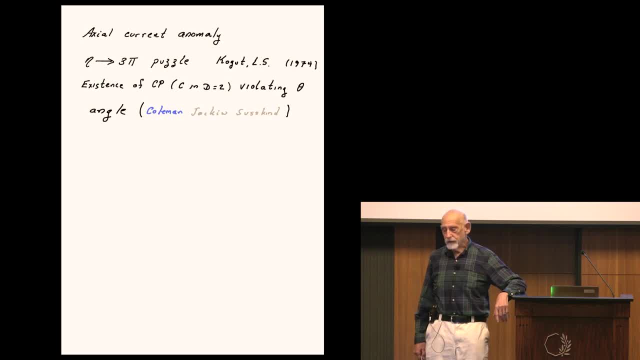 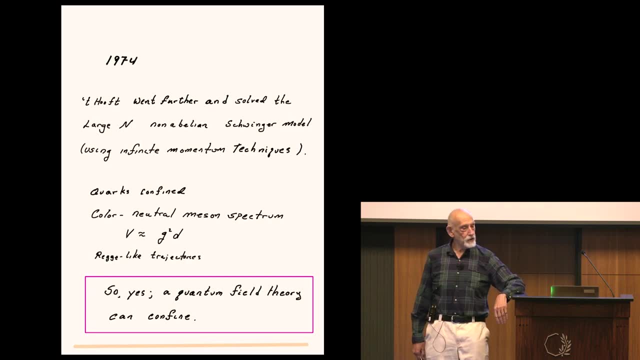 about this. the earthquake happened Asymptotic freedom. I was in CERN at the time. News came about: asymptotic freedom And boy, it shook the ground, Certainly shook the ground, my ground. that I was delighted. I said, wow, this is it. 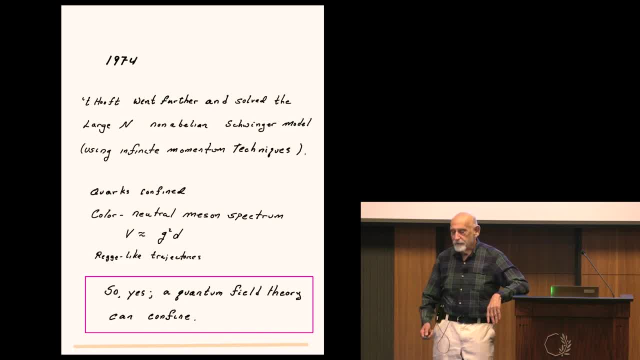 This is something great But, as I said, asymptotic freedom is a kind of bridge that bridges you from the weak coupling- small distance limit- to, let's say, the intermediate coupling at some moderate. It is not in itself the explanation or the mechanism of confinement. 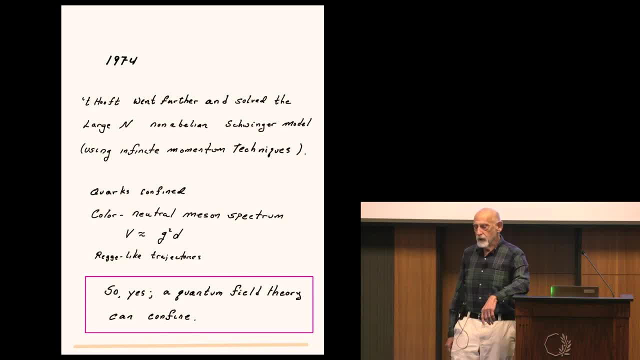 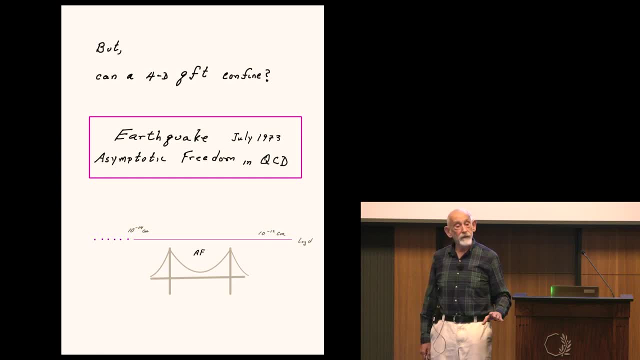 And so we began to think about that. Two things were key to generalizing the 1 plus 1 dimensional model. One was kinematical: The continuity of a flux. What's his name? Gauss. Gauss's rule That flux can only end on charges. del dot equals rho. 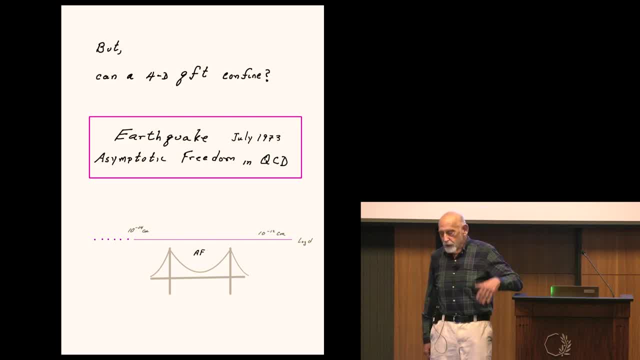 And the other was a new dynamical principle. And the other was a new principle of which much later I gave the name: nature abhors, a chromoelectric field. That idea appeared in papers by myself and John Kogut and very shortly after by Atoft. 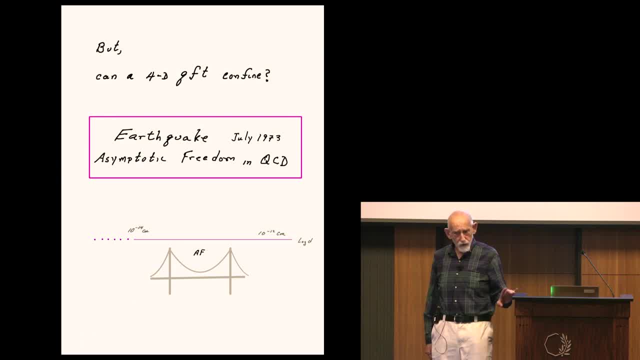 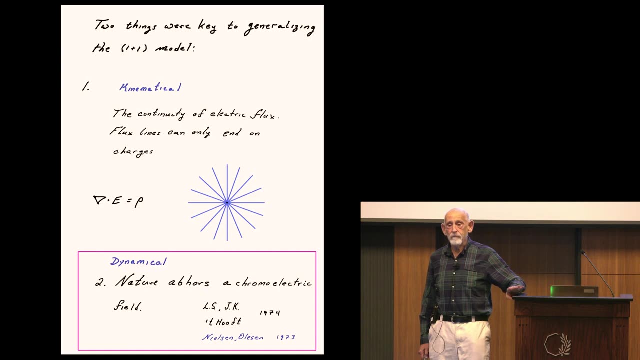 And it had a predecessor which was not really about core confinement. It was about creating strings from gauge theories, magnetic strings, not electric strings by Nielsen and Olson. What was the idea? What was the idea? The idea is, the vacuum is very unpermissive, with respect. 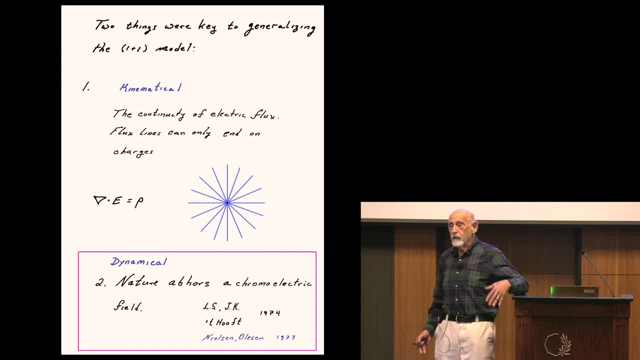 to allowing electric fields. The vacuum repels electric fields. The way Frank said it is that the electric fields tend to attract. Whether you say it that way or you say the vacuum tends to repel them, the picture is that the electric field lines 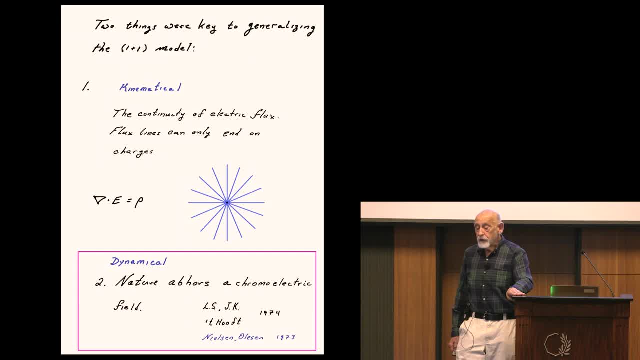 would form flux tubes. This was a new phenomenon. It was not just that couplings became strong. It was not just that couplings became strong, But new things happened. Among other things, it entails a spontaneous symmetry breaking of rotational symmetry. To understand why that's true, imagine a quark, a heavy quark. 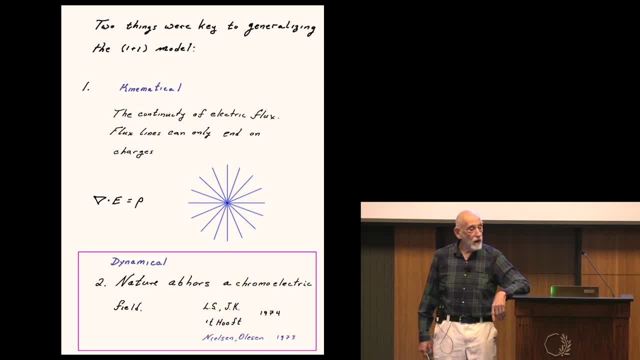 at the origin. Which way do its flux lines go? Well, they can go one way or they can go the other way. This is a spontaneous symmetry. breaking of rotational invariance. The spontaneous symmetry of rotational invariance has associated with it a rotation. 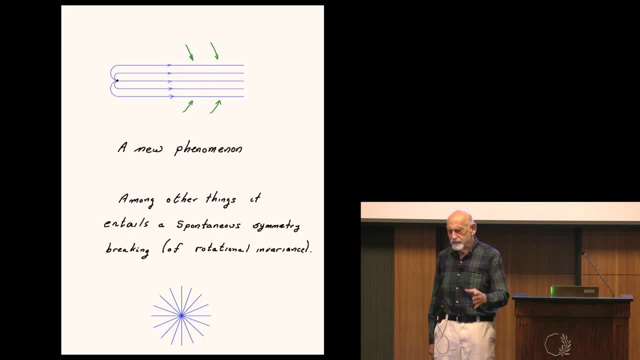 At the origin. the motion is non- causal. The motion and the motion are not so much olduğunu, but the formation of the motion. It's no longer a motion, It's not an atomic state, It's just a momentary event. 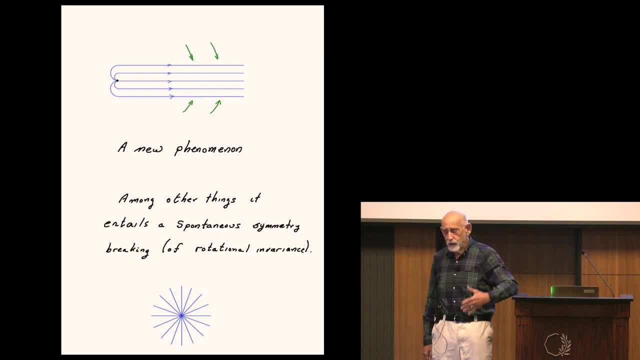 It's a momentary event And then what's very important is that you can don't have to deal with it. It's an instant state. It's an instant state And that just becomes a material out of the vacuum And it goes into thisけれvier state. 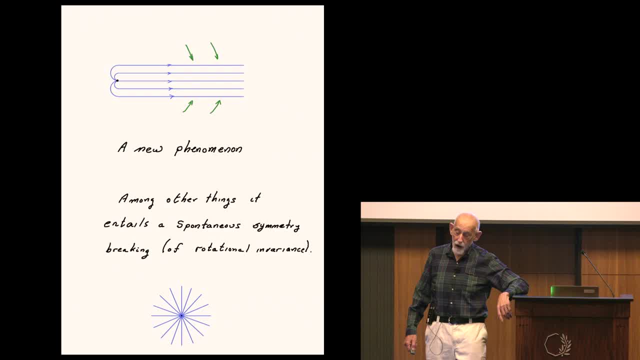 This is called the still state, a state in which the energy is AG1,, which is the horizontal dimension. If we look at this here, I show you where the energy gets released, But there's also a bracket. This is the stoic moment. 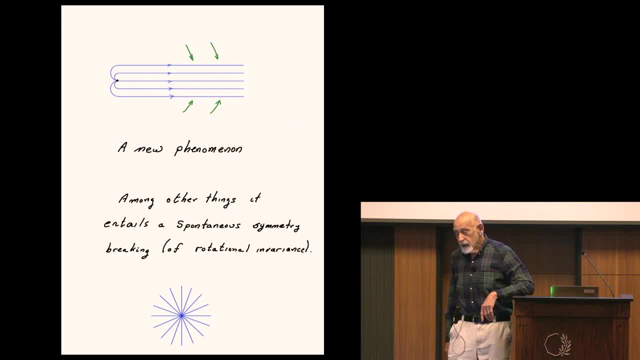 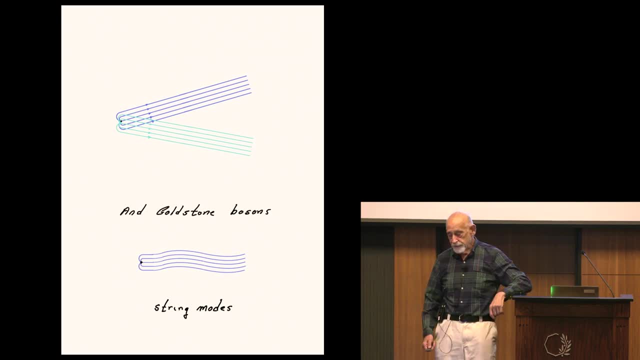 In the trochanterial state there's an influence can break by the production of light quarks But no free quarks And in fact if you have two outgoing quarks back to back with a lot of energy, the flux tube. 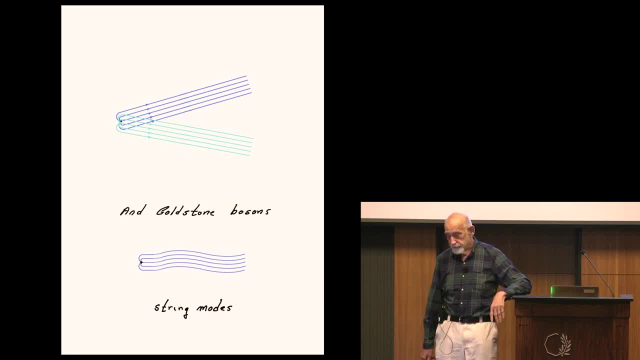 will break up into jets, jets of mesons. Glue balls should be able to exist in this theory. Just as in strings there are closed strings and open strings, glue balls should be able to exist, So again can a field theory- now I use the word field- 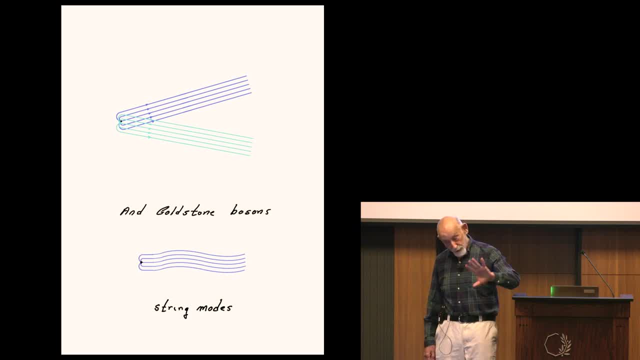 theory, not quantum field theory, because it's a little too hard to answer this question about a real quantum field theory. But can a semi-classical field theory behave this way? A model was put forward again John Cogan and myself. 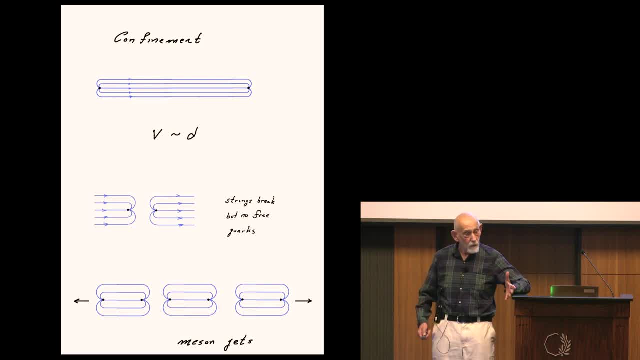 and, shortly after a tuft, a construction of a field theory which does this. It's based on the idea of a polarizable vacuum: Epsilon. here is the local dielectric constant, sometimes called the permittivity, And the interesting thing is that the sine of epsilon minus. 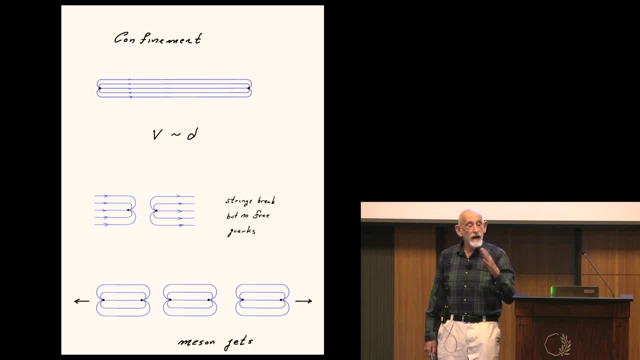 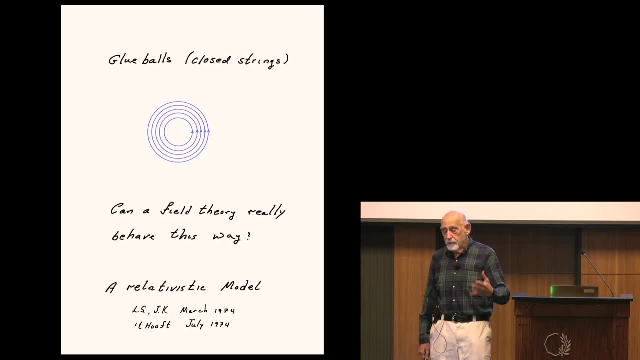 1, where the epsilon is greater than 1 or less than 1, is related in a certain sense to the sine of the beta function in QCD. If you're trying to model an abelian gauge theory, then epsilon is always greater than 1.. 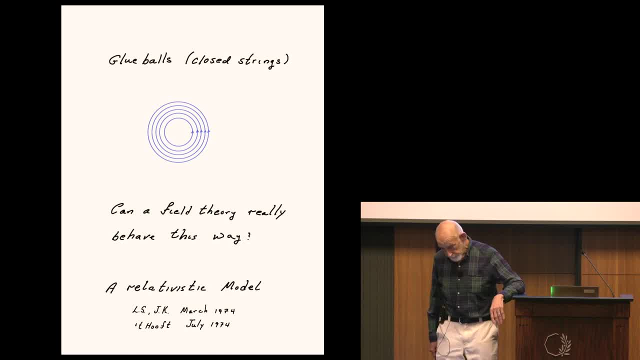 That's just the usual Debye screening of a charge In asymptotic freedom. Roughly speaking, it behaves as if epsilon were less than 1, anti-screening. So we built a theory with this epsilon field. Epsilon becomes a field now. 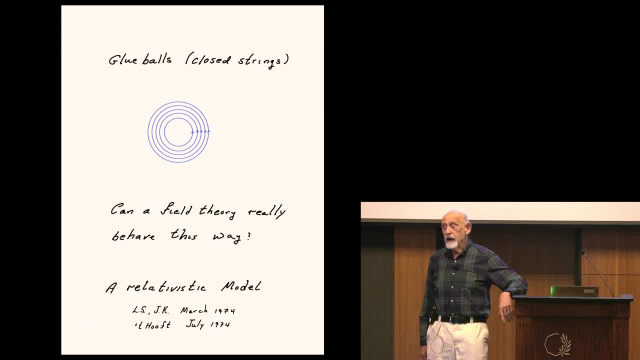 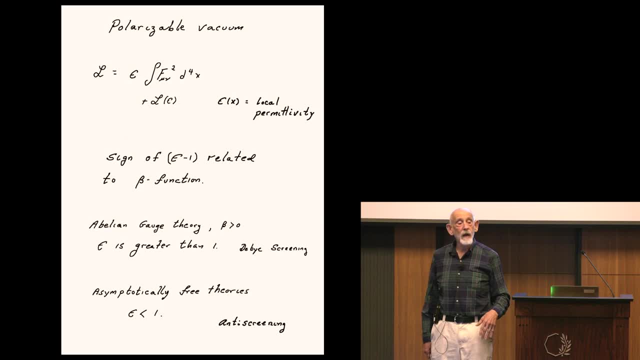 And assumed- and this is an assumption, of course- that whatever the Lagrangian as a function of epsilon is, it favors small and even vanishing value of epsilon. You can solve the semi-classical equations for this And what do you find? 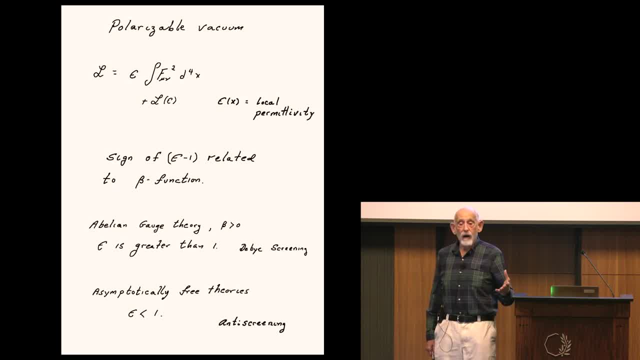 You find very near the charge. You can find very close to the charge. There's a region of more or less normal vacuum epsilon of order, one in which the charge spreads out in the same way as it would in a weak in electrodynamics, but far away. 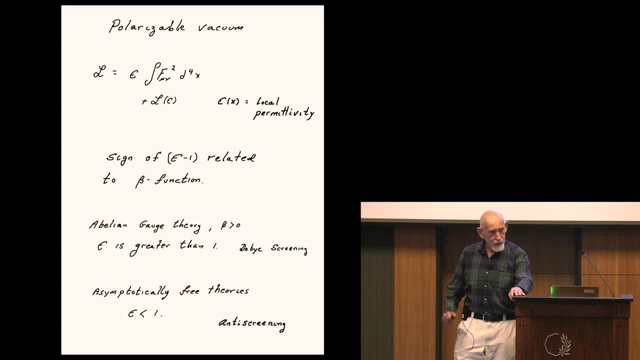 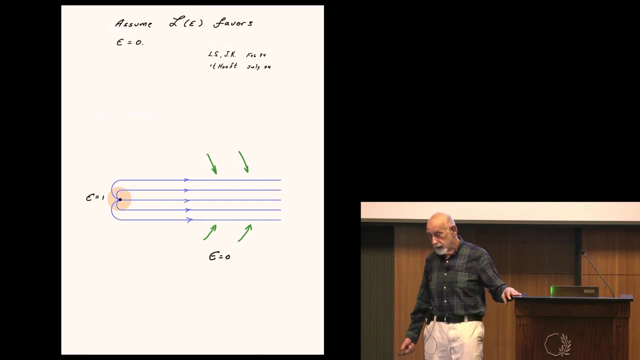 excuse me, it forms these flux tubes. Nature abhors a chromo-electric field. which are close together would be surrounded by a normal region, have a Coulomb force between them Two quarks far away, would have a linear growing potential. 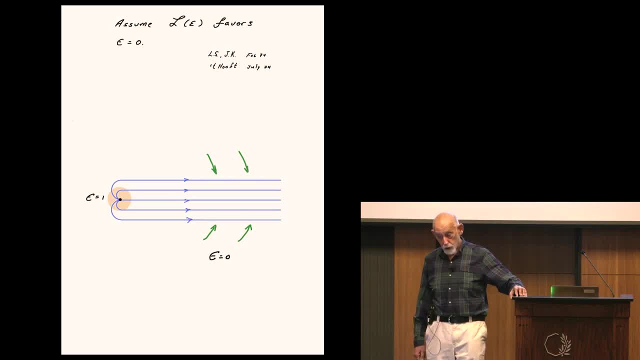 Then, in February 1974, another quake Wilson, building on the ideas, the statistical mechanics ideas of Wegener, in 1971, created Euclidean lattice gauge theory. Thank you, That's great. Now, I think, to this audience I don't really have to explain in great detail. 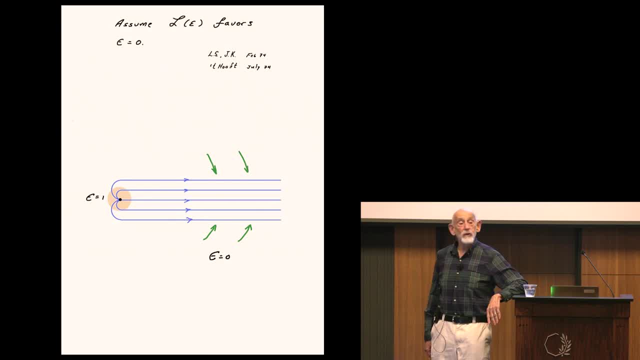 In a weakly coupled gauge theory, the Wilson loop, that's the amplitude for a quark trajectory going in a loop- is proportional to E, to the minus I, the action, and the action is proportional to the perimeter. This is of course very famous, the Wilson loop behavior. 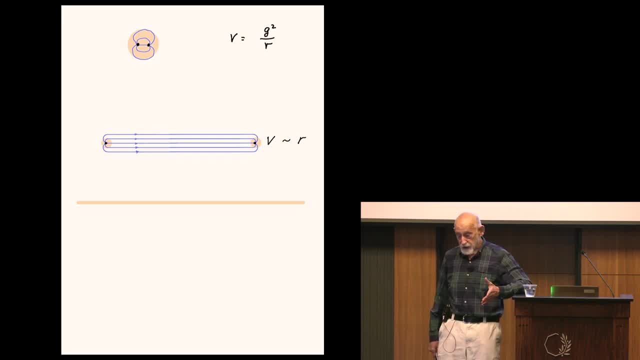 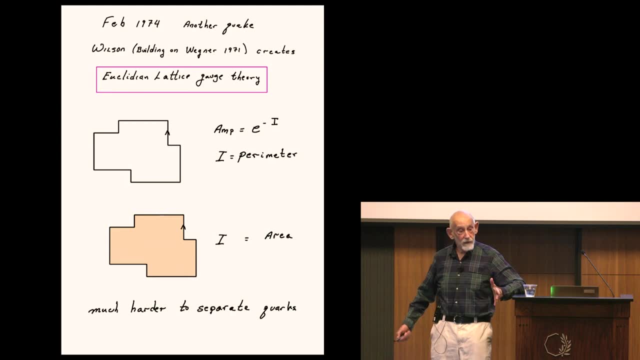 But in the strongly coupled regime of the lattice gauge theory the action behaves like the area That makes it much harder to pull quarks apart. In fact, it's easy to see that it basically says: you can't pull them apart. Much harder to separate quarks. 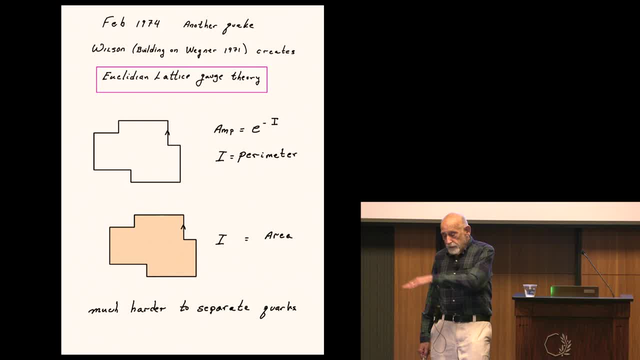 What was its relation to the string theory ideas? Well, if you cut through, this was Euclidean gauge theory. If you cut through it, the Wilson loop, you would see what looks like a string. A string, It's just a cut through the world sheet. 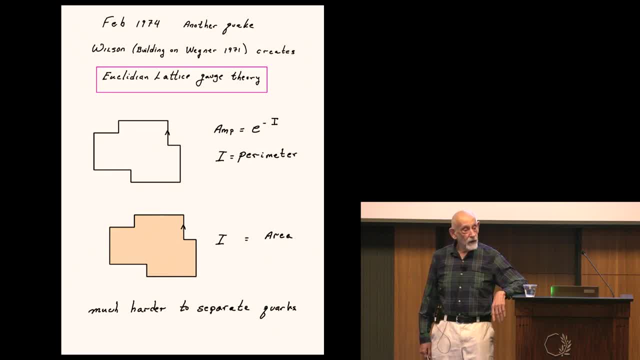 And it's a string. I had a long conversation with Wilson about this. He had never heard of string theory. in fact He was very delighted by it and extremely encouraging to pursue the analogy with string theory. But the question came up: can lattice gauge theory be used for real-time processes? 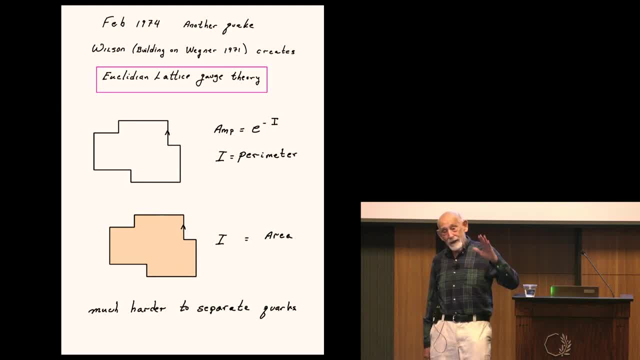 Not if it's in its Euclidean formulation- The idea that you can analytically contain- you know things as difficult as I see Frank smiling- That's not something that's feasible. You really have to have a real-time formulation if you want to do real-time physics. 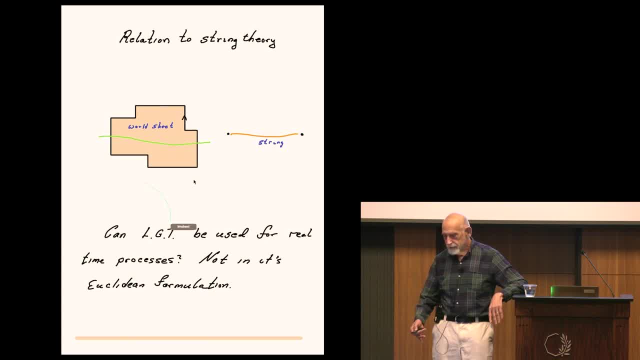 Why isn't this going? Oh, there's something up here. What is it? Help, There's something on the screen here. I can't, I don't. they took my glasses away. I can't even, I don't know. 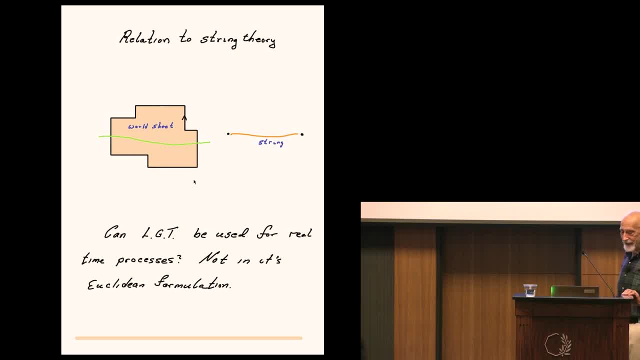 Remember I get an extra three minutes. Try now. Okay, What was needed was a real-time Hamiltonian formulation of the gauge theory. Hamiltonian lattice gauge theory. John Colgate and I started to think about it up in Ithaca. 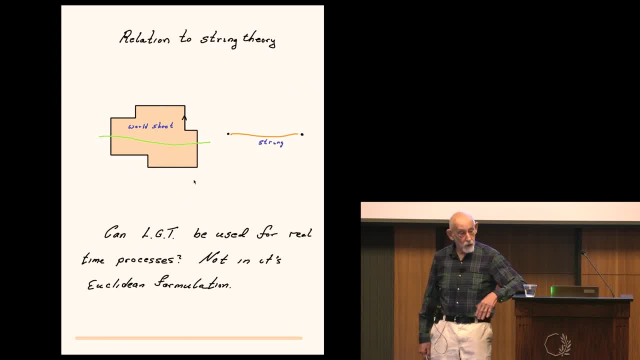 We were up in Ithaca. I was visiting him there and talking a lot to Ken Wilson, But one night, I think, I just worked out. it took one night to work it out. You'll probably know a good deal about it. 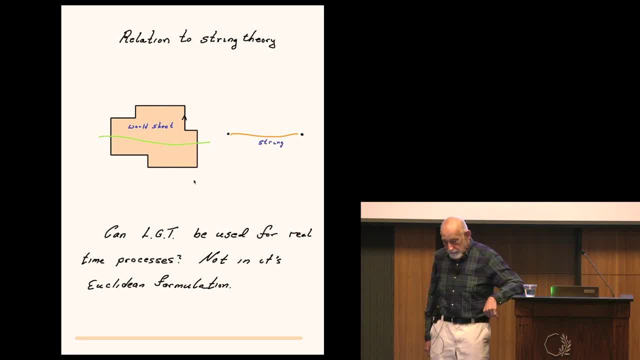 Space is a lattice. Time is a continuum On that spatial lattice. electric fields live on links, Magnetic fields live on plexi And quarks live on sites. I've written a Hamiltonian down below. It looks much more complicated than it is. 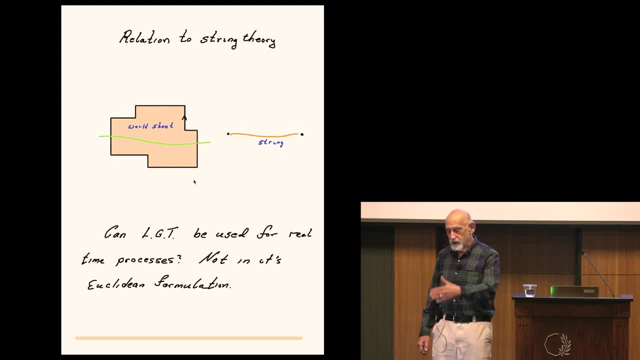 It's really very simple. It has an electric field term that starts, the first term, G squared, proportional to G squared. There's a magnetic field term, which is the 1 over G squared term, And then there's the quark kinetic energy, together with 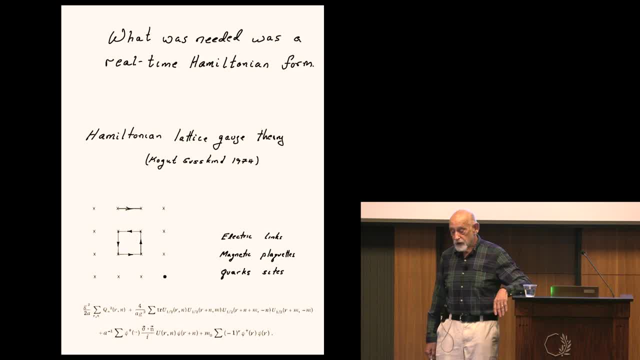 it's coupling to the gauge fields, And that's G to the zero. What was interesting again, as Frank pointed out, is that in the strongly coupled limit the chromoelectric field is quantized. And not only is it quantized, but in the vacuum. 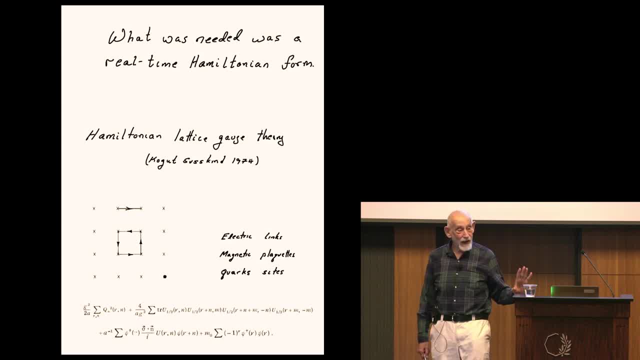 it is equal to zero. Now, it's not zero in the sense of expectation value, It's zero in the sense of zero. The vacuum is completely free of electric field fluctuations in that limit, And indeed nature abhors an electric field. 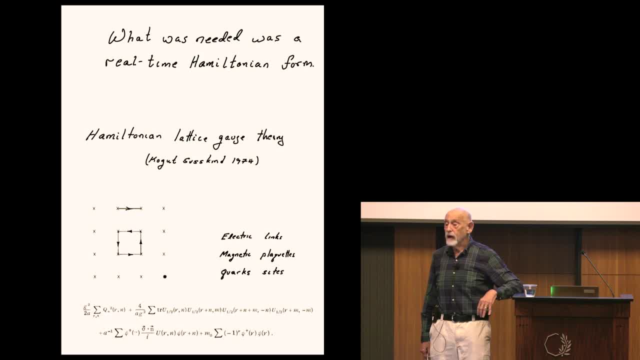 If you had a pair of quarks, because of the constraint of Gauss's law, they have to put out some electric field. They'll put out the electric field in the form of quantized string of electric flux which will go from one quark to another. 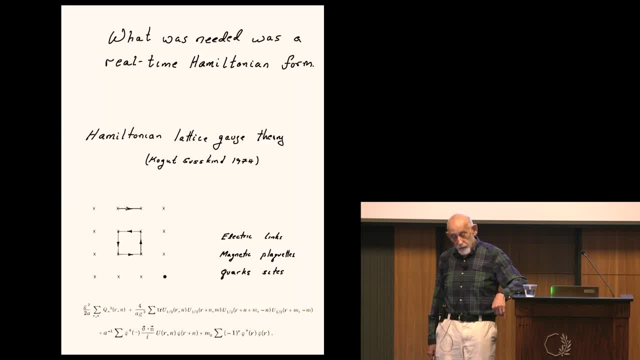 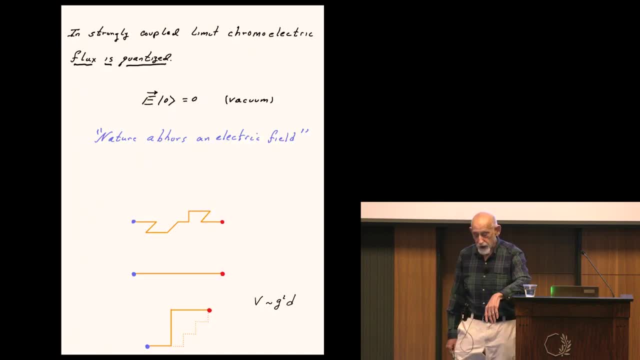 It can go along any route, But of course the cheapest route of the cheapest energy is to go in a straight line Again, the potential energy being proportional to separation. forget the next picture. I won't do that. I don't want to ignore it. 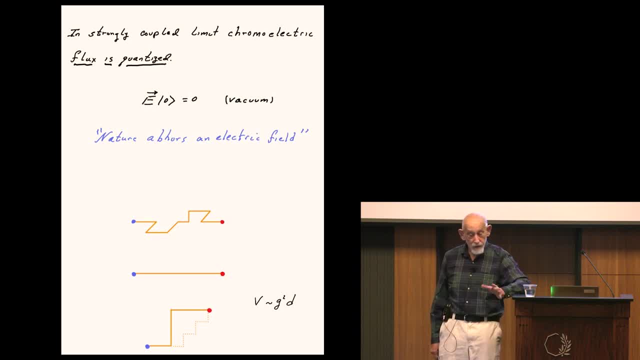 All right. So in principle, I don't know to what extent it's ever actually been done. Hamiltonian lattice gauge theory can be used for real-time processes. I don't know why there's a question mark there. No, that's an exclamation point. 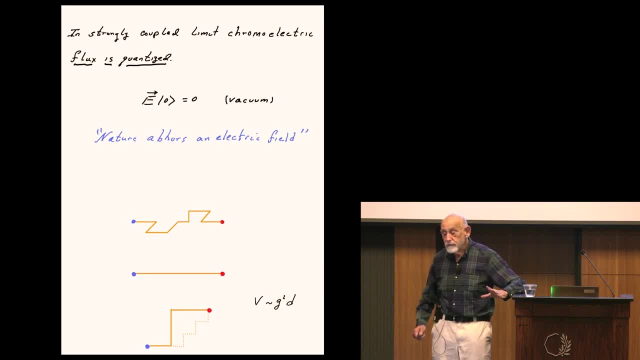 Decays, scattering, meson, jet production in principle, E plus, E minus, interhedrons and so forth. Now the Hamiltonian, as I said, comes in three. It comes in three terms: a strong coupling piece. 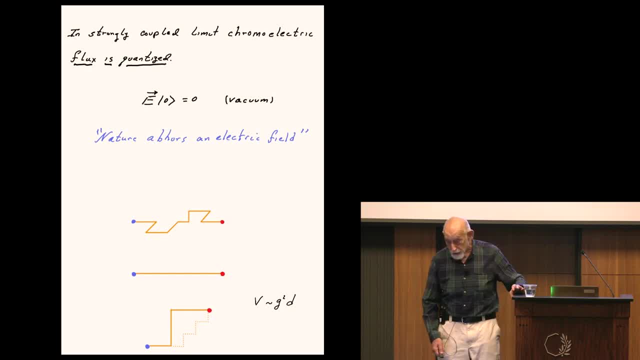 proportional to G squared, a piece proportional to G to the zero, and another piece proportional to one over G squared. This strongly suggests to think about perturbation theory in powers of one over G squared. What does it do? It creates little fluctuations of electric field. 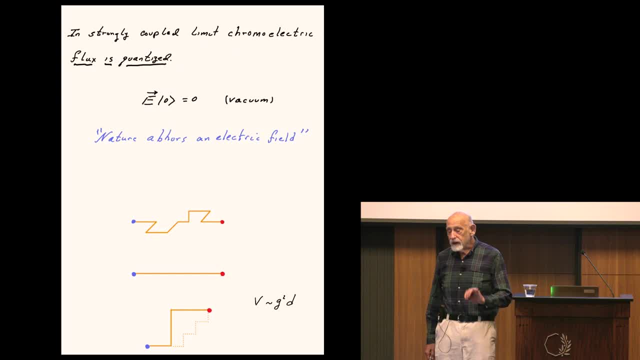 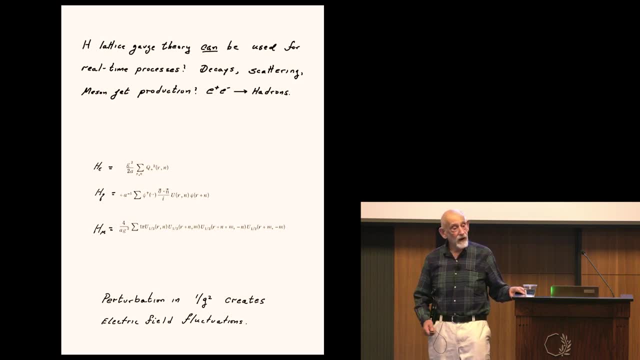 removes certain degeneracies. but, especially interesting, it allows systematic computations of masses, moments, things like GA over GV, that's the axial vector, coupling constant F, pi, other kinds of quantities which you can now try to calculate by perturbation theory in powers of one over G squared. 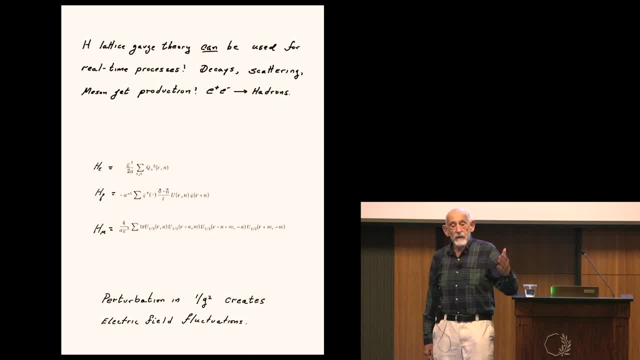 I'll call one over G squared X. How do you? what can you do with perturbation theory? Well, you have a couple of terms in perturbation theory. In principle, we're really trying to continue it to small coupling. Why? 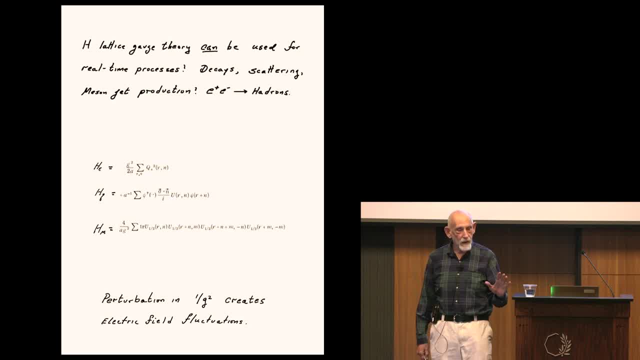 Asymptotic freedom tells us we should really calculate dimensionless quantities at G equals zero, for reasons that have been explained. How can you continue your answers to G squared equals zero? Well, a convenient tool which you would be perfectly right to be skeptical about, but still it works in some cases. 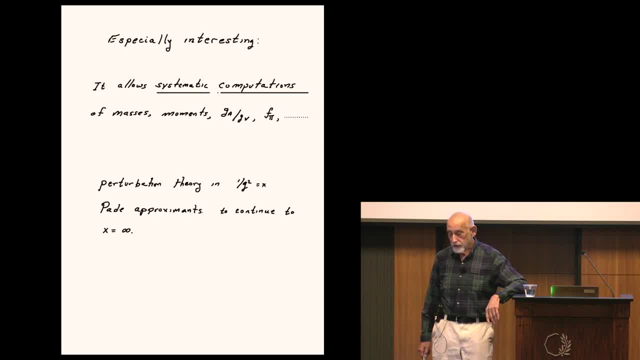 are Padde approximants. to continue to, X equals infinity. Kogut, myself and Don Sinclair applied this to the pure QCD, which would be a theory of glue balls, and calculated a glue ball spectrum. At that time there wasn't much in the way. 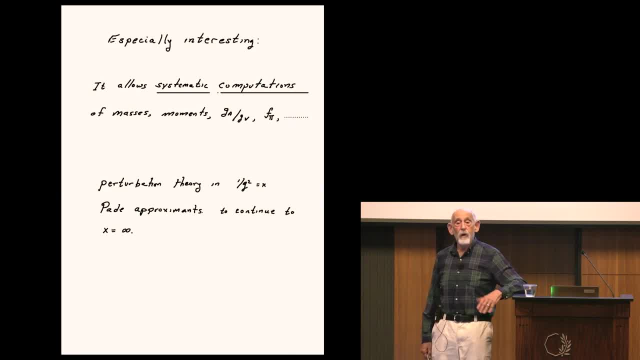 of experimental information about glue balls, so it was more an exercise and it was an easier exercise than including quarks. We calculated a glue ball spectrum. I think it's a respectable glue ball spectrum. But more interesting was to apply these ideas to real mesons and baryons. 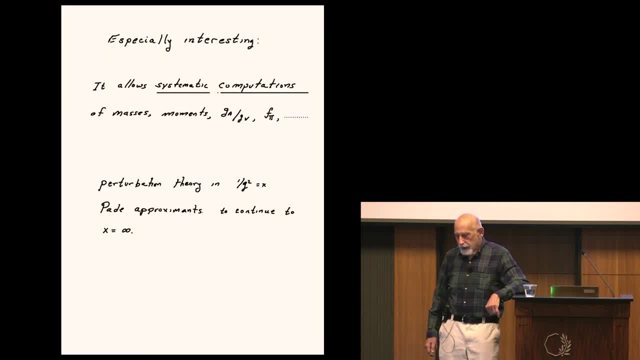 That took another year of work. It was hard work. The reason there were seven authors on the paper is because all this was done by hand, No computers at all. We didn't even trust ourselves to calculate correctly, so it was important to have backup from different people. 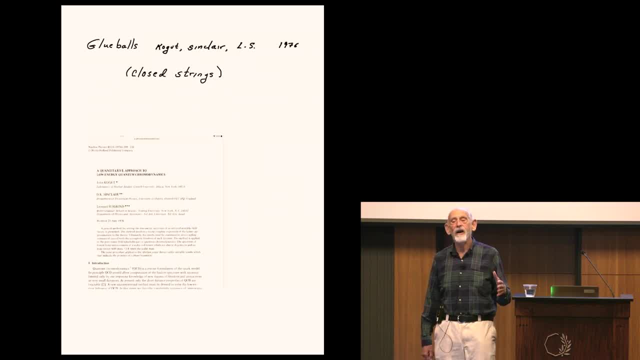 doing the same calculations. There was something like about 300, or maybe it was 400 separate little contributions coming in perturbation theory for even the same thing. In fact, we did this in the simplest kind of particles, In zeroth order, with no correction. 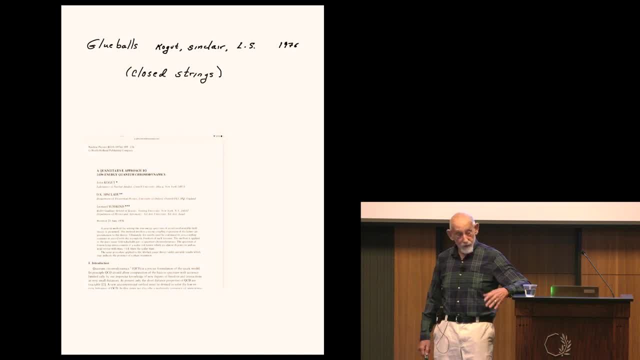 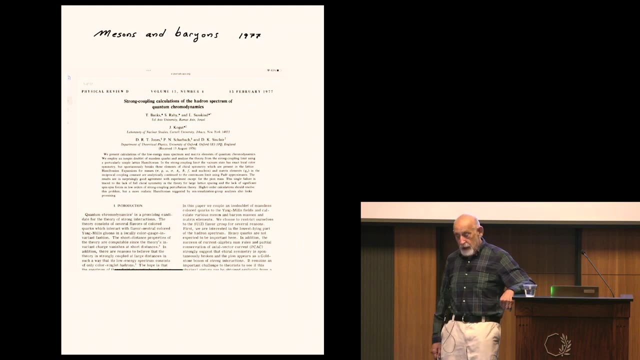 the strong coupling limit? the answer was that with the particular setup, we had staggered fermions. the mass of mesons divided by the mass of nucleons was too big- 1.25.. The axial coupling was also much too big- 3.. 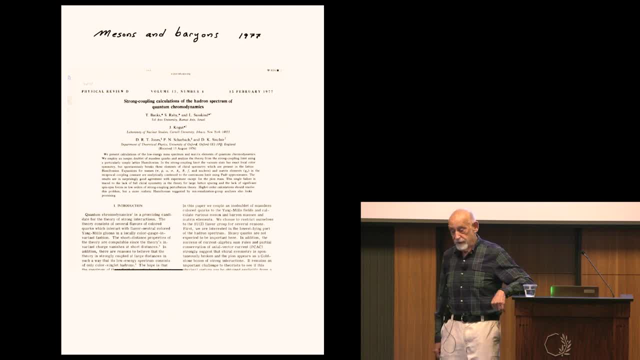 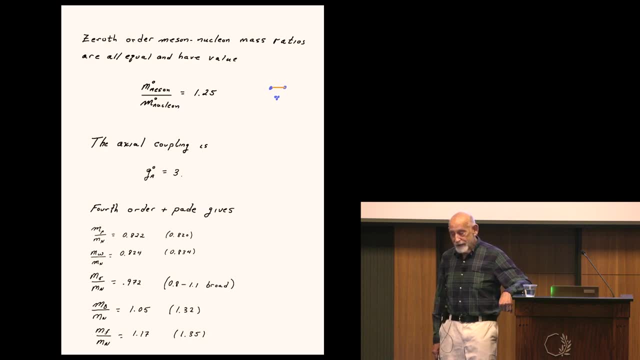 Forth-order Padet approximants gave answers: M rho: over 2.25, over m-nucleon 0.822, that's to be compared experimentally with 0.82, now that's an accident. there's nothing to be gleaned about the fact that this is a good to two decimal places. 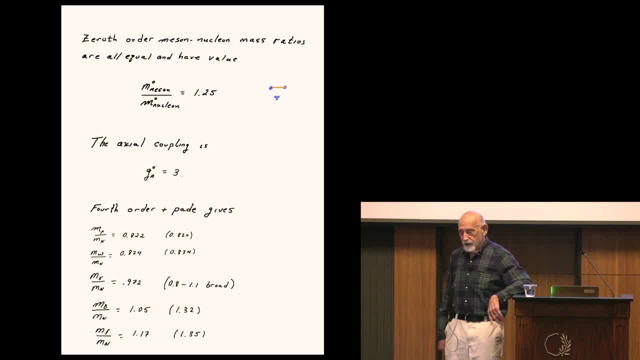 accident. m-omega is also very good. there's a thing called the sigma resonance, which is not a resonance, it's just a very broad fat blob, but it's nominally somewhere between 1.8 GeV and 1.1 GeV. it came out in this theory at 0.972,. there's something called. 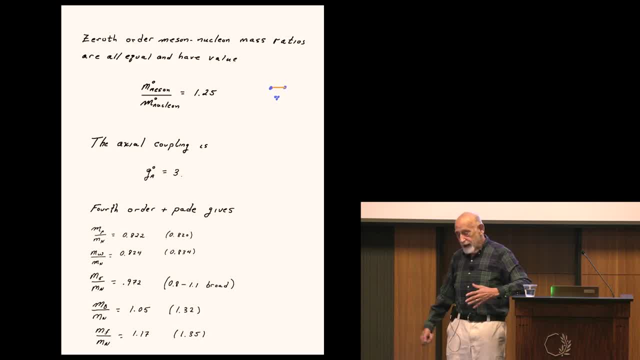 a b-meson which I can't quite remember what it is. it came out at 1.05 as opposed to experimentally 1.32, there's an F. I think the F is an excited state of the row. anybody remember? 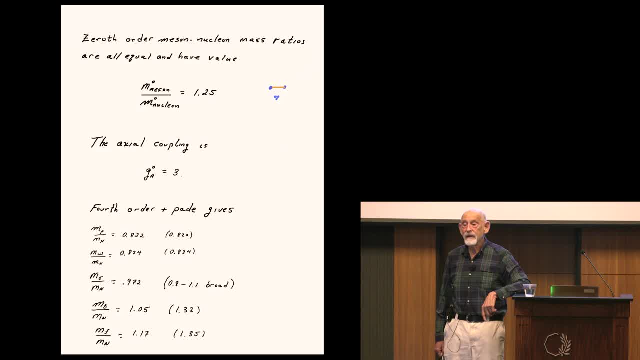 What? It's been true, I noticed it's higher than the test. Ah, Yeah, Right, you were just waiting to say that, right, yeah, Came out pretty darn well. the A1, which is an axial vector meson, came out rather well. 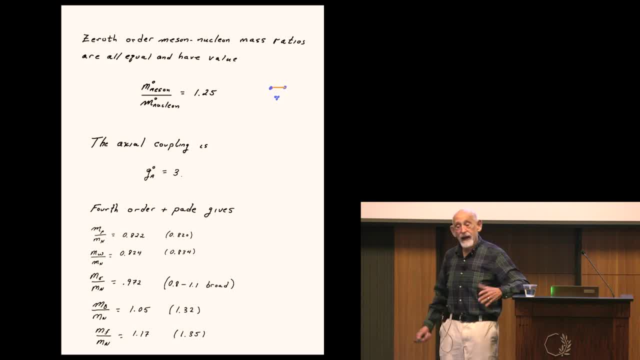 and GA went down from 3 to 1.8, that, I have to say, we considered good, very good. the pion, by contrast, was not good. it refused to move away from this. well, it moved away from 1.2 to 1.3.. 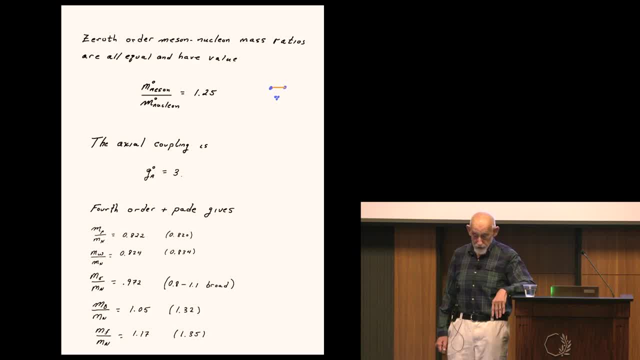 Well, it moved away from 1.25, but it wasn't being split from the other mesons. That is when, or somewhere before that, Ken Wilson had said: beware of the pion. I still do not really know what to make out of this. why the pion? keep in mind the axial. 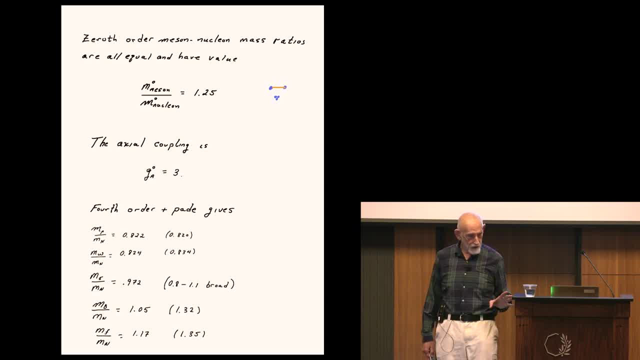 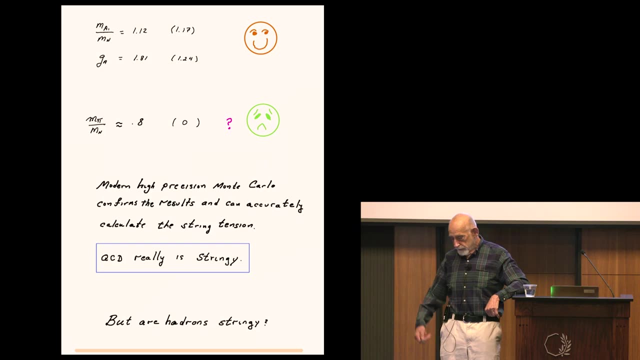 current conservation is a discrete symmetry on these lattices, and it just seemed that it was hard to get in this order axial things to work out well, So I really don't know what. the what, how good did we do? very, very good for most things. 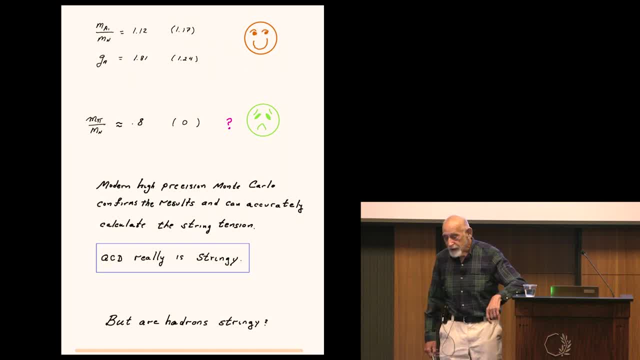 and really crappy for one thing. well, I don't know what to make out of that. Anyway, modern high precision Monte Carlo confirms the results and can accurately calculate- which we also could have calculated, things like the string tension Upshot. 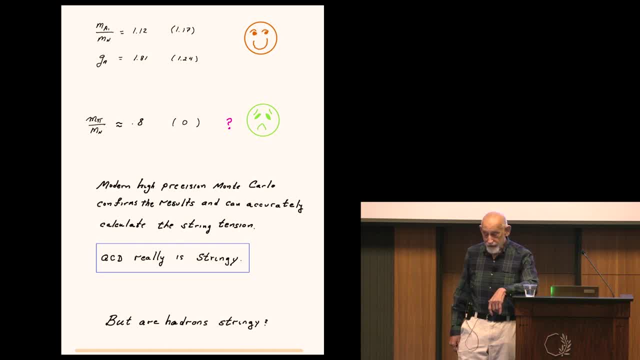 QCD is a stringy theory. It is a theory of stringiness. I won't say strings, because strings already carries a context of certain mathematics. but they're certainly stringy, like Turkish taffy. you pull it apart. But are hadrons stringy? 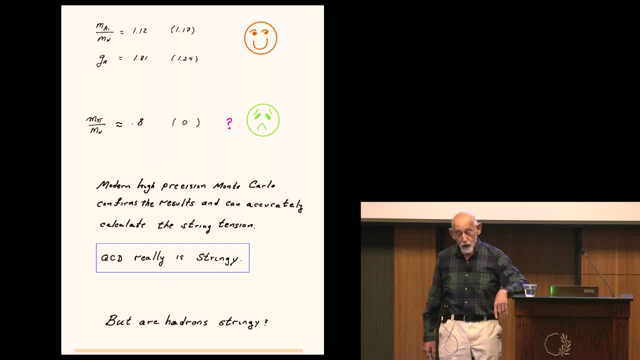 QCD is stringy. Are hadrons stringy? That's an experimental question. I think the best experimental evidence still probably comes from linear regis trajectories. Those linear trajectories that Chu and Frouchi had somehow conjured up from nowhere are real. 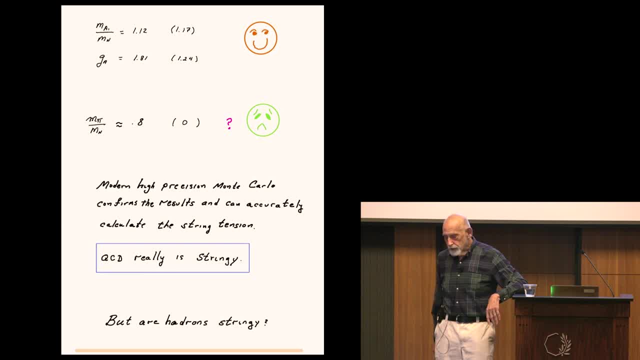 This is the Rho trajectory. has one, two, three, four, five, six, six states on it, and boy do they lie on a line. This is the omega. Omega is another vector, meson also a good straight line. 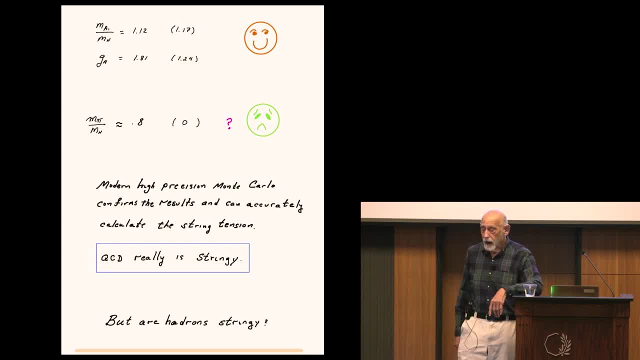 This is the delta, three halves, The baryon part. Okay, The baryon partner, the symmetric baryon partner of the baryon itself, of the nucleon, also lies on a straight line. Here's a strangeness: one baryons. 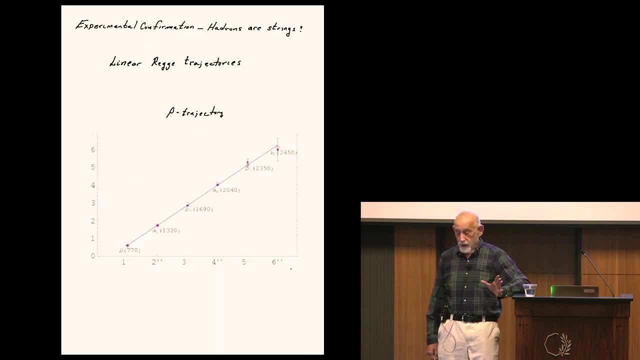 I got this off the internet. I found them. Question: What happened to the daughter trajectories? Why don't they appear? Ask me later. What about pion jets? Is that another source of experimental information? But before we go there, Okay, 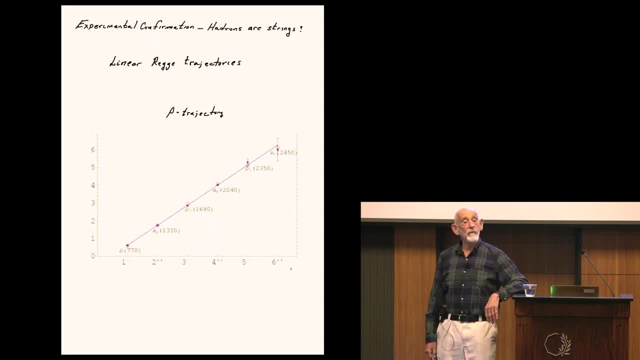 Let's talk about the magnetic properties of the vacuum. One theory of confinement which I think is a legitimate theory of how confinement can happen, is magnetic monopole condensation, a transition from having monopoles to having the monopoles go massless and at some transition point, the confinement transition the monopoles. 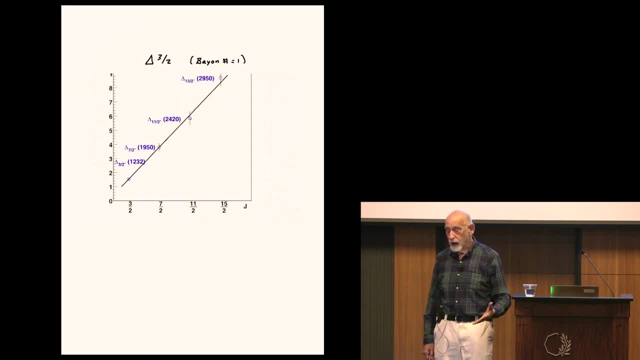 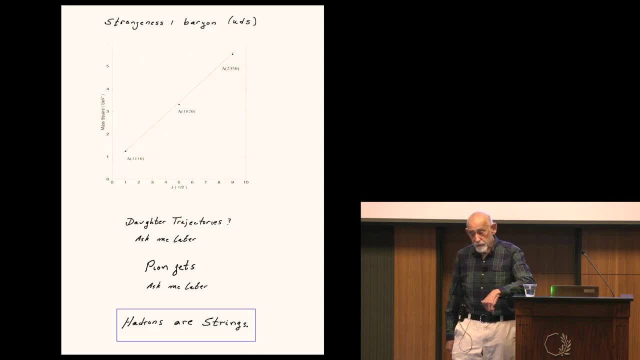 condense. That would be associated with what I would call magnetic condensation. Okay, That would be associated with what I would call the electric Meissner effect. That happens in abelian lattice gauge theory, a transition between the two. It happens in certain supersymmetric versions of QCD. 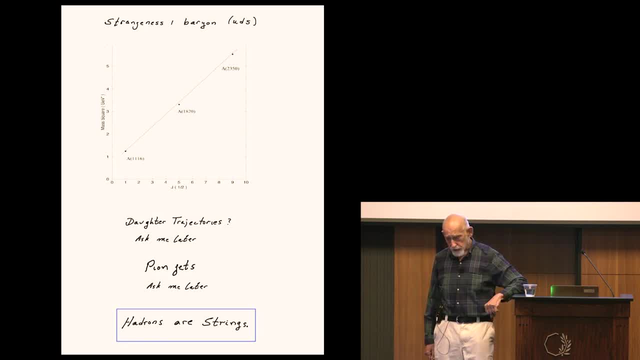 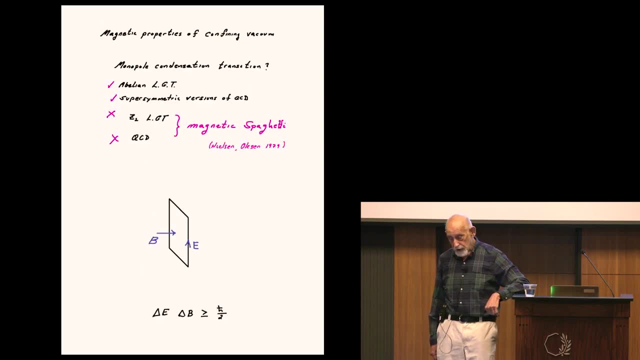 It does not happen in other theories which also have confinement transitions, namely the Z2 lattice gauge theory, And I don't believe it happens in QCD. Instead, I think what happens is something that Neil said: Okay. I think what happens is something that Neilson and Olson somewhat later called magnetic spaghetti. 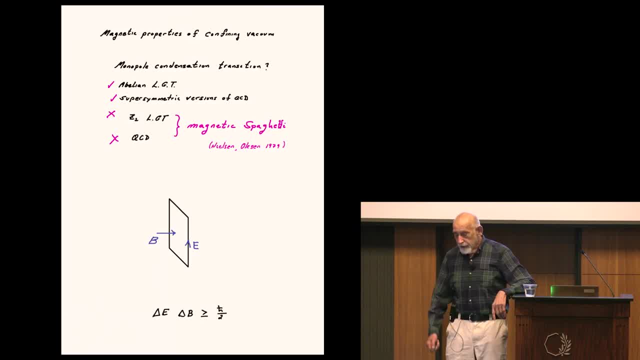 So I'll briefly tell you what magnetic spaghetti is. There's a plaquette. I've drawn a plaquette. The magnetic field is associated with, roughly speaking, the line integral of the vector potential around the closed loop, or the product of the unitaries going around the closed loop. 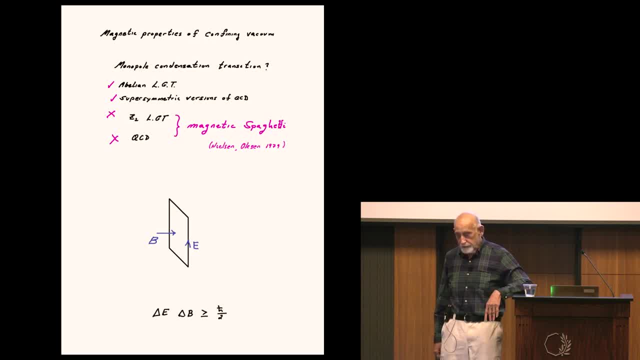 And the electric field is associated with the edges. The electric field and the vector potential are canonical, Okay, Okay, So what does this mean? Well, the magnetic field has two canonical conjugates. Because they're canonical conjugates, there is an uncertainty principle. 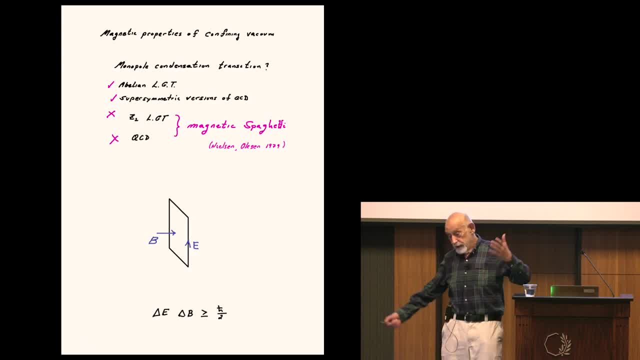 Delta E, delta B is greater than H bar over two, Because nature abhors a chromoelectric field, whether it be just because we made it up or because we're coming from lattice gauge theory, it says that the magnetic field is wildly varying at strong coupling. 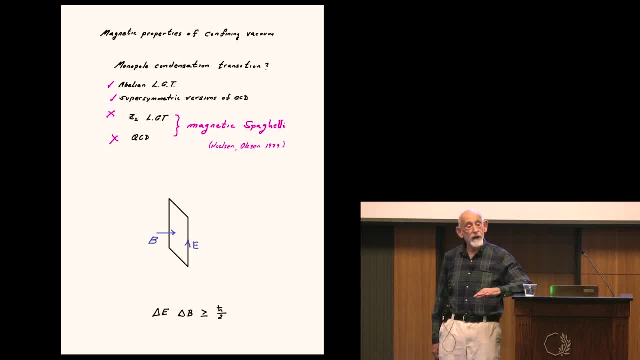 Okay, Okay. has a wildly fluctuating magnetic field, subject only to the constraint of flux continuity. That is what Nielsen and his collaborator called magnetic spaghetti. I think that's actually the right magnetic picture, not the picture of magnetic monopoles in this case. 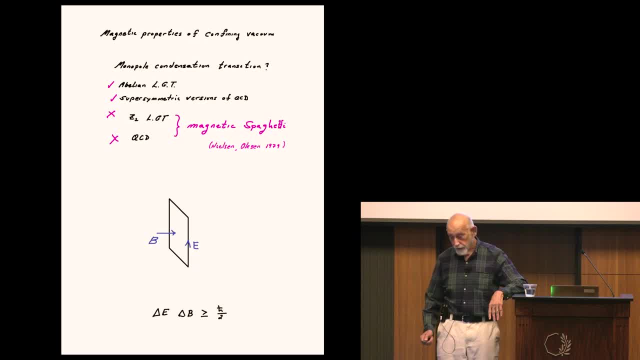 although magnetic monopoles are a possible explanation of confinement. The other thing I would mention is the importance of Etouft's discovery of large N and planar diagrams. We know the story there. The most interesting thing at the time for me was that the planar and non-planar diagrams 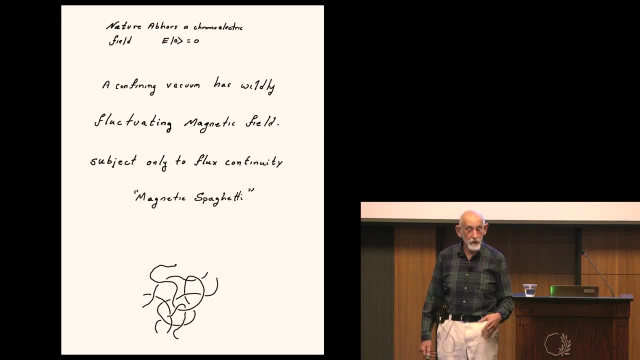 organized themselves into these topological classes, which were in one-to-one correspondence with the topological classes of world sheets. in string theory, By now the Etouft large N expansion has become a central part. It's a central part of so many things. 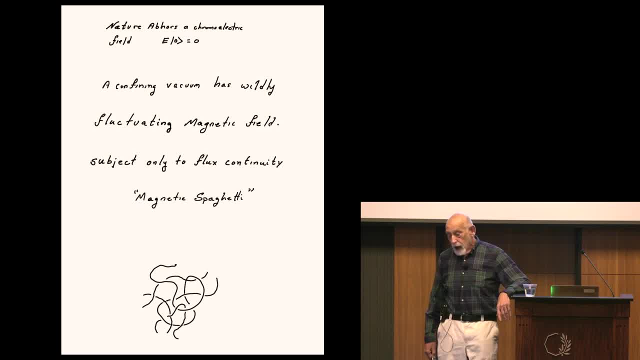 that I don't think I need to tell you, including black holes, incidentally- And that is the story that I was going to tell you- about confinement, the confinement mechanism. Now, the confinement mechanism was a genuine discovery. It didn't just happen. 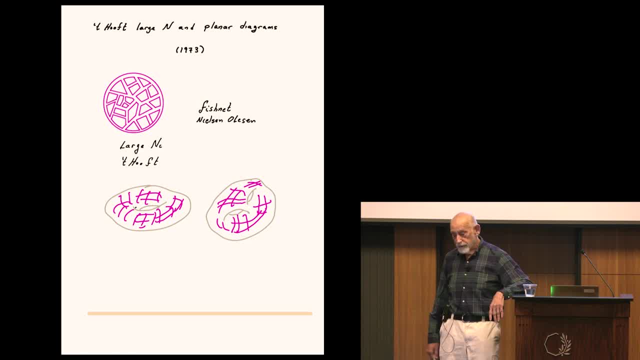 It took place over a period between 1969 and 1975,, I would say. But the reason I talk about confinement is because of the people behind it. I think they have a little bit of a history. So we're talking about the fact that the city 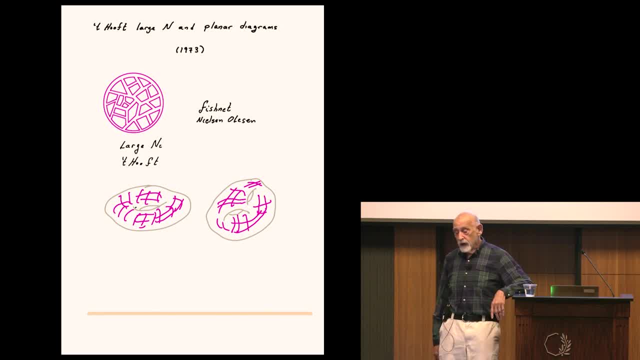 was created in the 80s, in the 1950s, when the city was just an exhibition space that was held for the time being, And we're talking about the same theme, So it's the movement of the city, And that alone is so interesting. 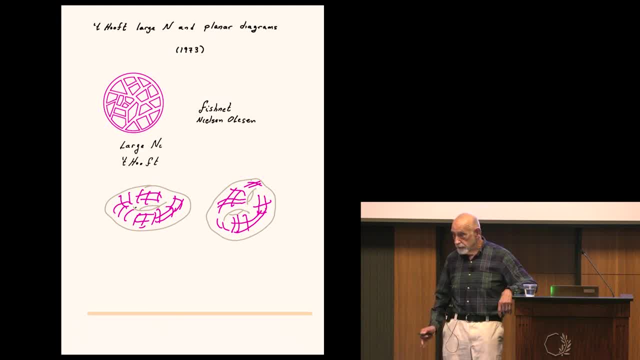 And I don't mean to be well verbatim or the opera, because that's what we're talking about. It's not an attempt to be personal, To make people think, It's not something that you do when you're dead. 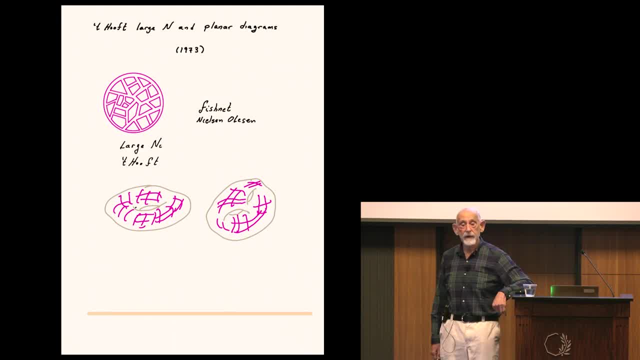 It's something that you do when you're dead. You're supposed to be doing it, but not only that, But it's not like that. Let's see anything else. Ah, how much time do I have? Okay question is: what happened to the daughters? 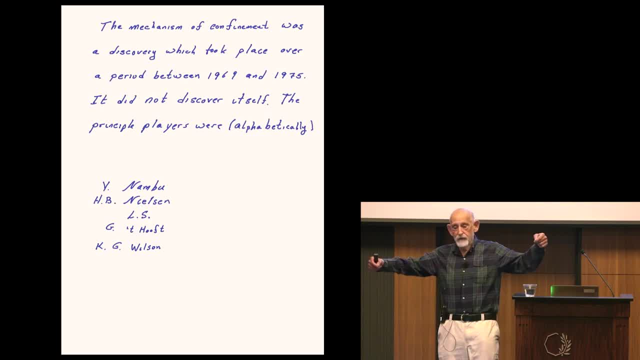 The leading trajectory in a string theory is just a straight string rotating about itself like that. It's very straight and therefore it doesn't tend to intersect itself very much, if at all. The subleading trajectories, the daughter trajectories, are generally configurations of the string. 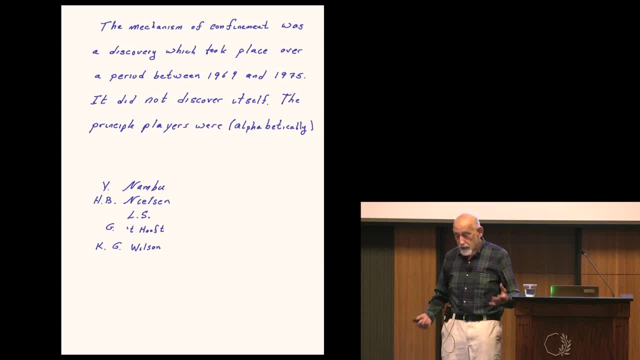 which are more crowded, more messy, Lots of opportunity for crossing and splitting, Lots of opportunity for decay and distortion of the spectrum. So it's not too surprising, I think, that the daughters, to the extent that they exist, may not look have this pristine, linear, rigid trajectory. 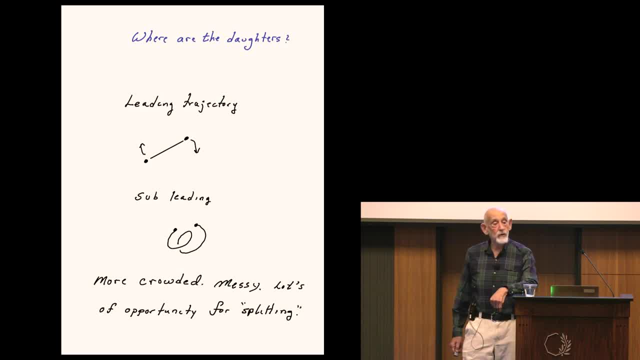 I think that's natural. I think that's natural and normal. Let me also mention jets. Jets are another source of potential understanding or potential string theoretic behavior From asymptotic freedom. we know that when two high-energy particles collide, that quarks can be produced, at first sight, freely. 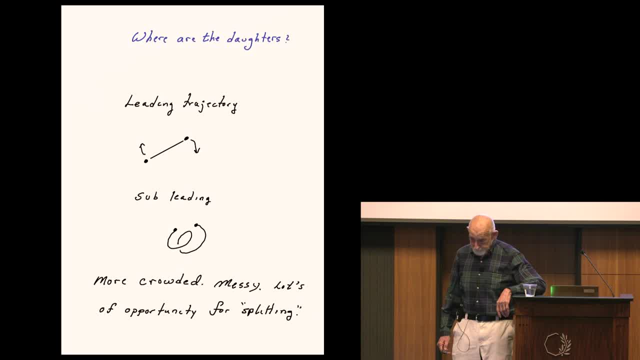 at very high energies. Those quarks go off with very high energy, But of course we know that this is subject, that this is subject to the confinement mechanism, And so what we expect to happen is long flux tubes connect them If there were no dynamical quarks or light quarks. 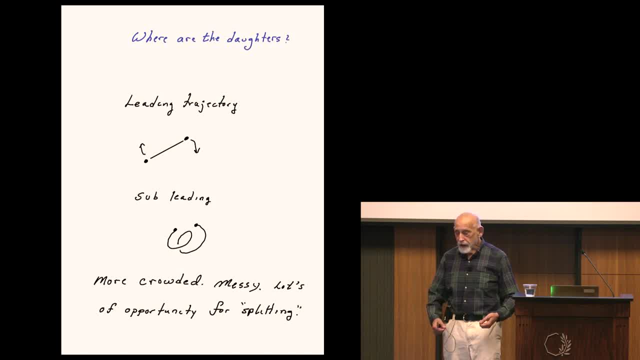 then I think, as Frank said- or maybe it was Michael- all that would happen is it would go back and forth, back and forth, back and forth. But what really happens because of the light quarks is they fragment into these jets. 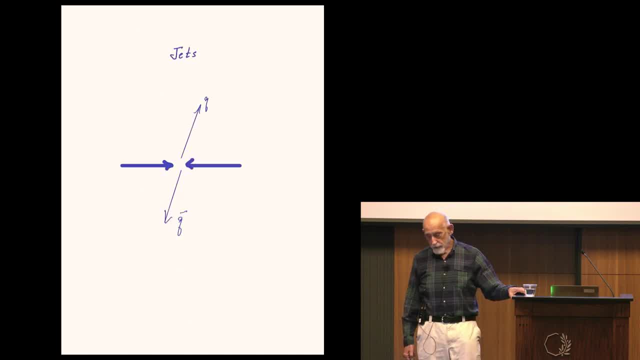 The jets are a real thing. I don't know if this still exists in the literature. Feynman did a very interesting analysis, very elementary and simple analysis, of how the jets reflect the quantum numbers of the parent quarks that created the jets. 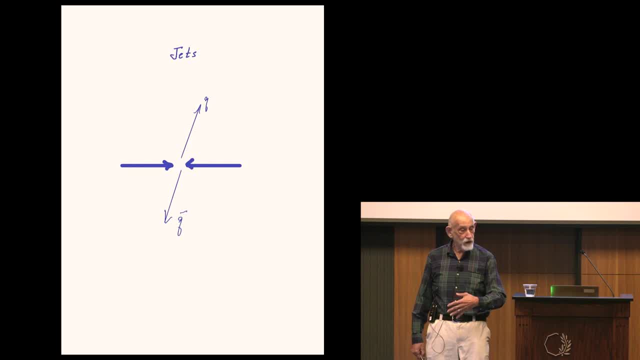 If it still exists- I couldn't find it because I can't find the Laszuch Summer School lectures, But if it still exists it's very pretty, it's very nice. Not quite exactly right. It shows you how the jets really reflect the physics. 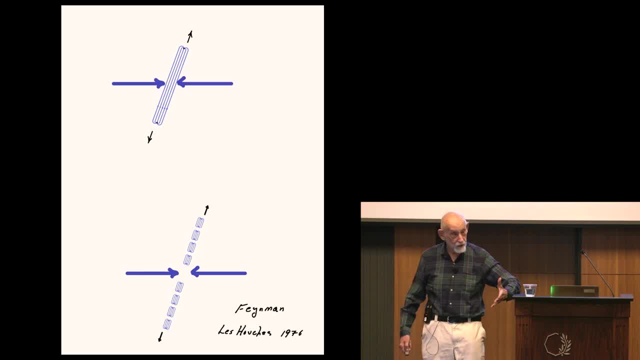 of the production of quarks and the production of, and the mesonification of the jets- mesonification. Okay, I think that that's yeah, that's it. That's all I had to say. Thank you, Yeah. for me this is something of a homecoming. 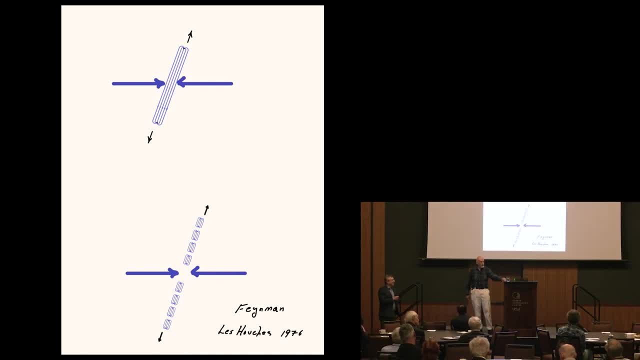 Yeah, for me this is something of a homecoming. Yeah, for me this is something of a homecoming. I think I feel sort of like Odysseus coming back to Ithaca after- well, in this case, 43 years. 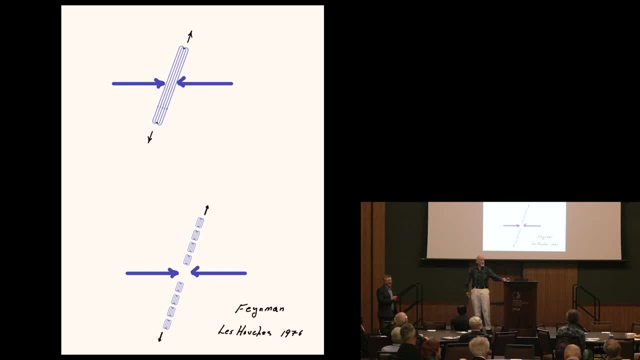 And it feels good. It feels like I'm home again with my first love, which is all of you people. Do we have any questions? Comments? So one thing you didn't mention is your work on repartons and the connections to repartons to ideas about thinking. 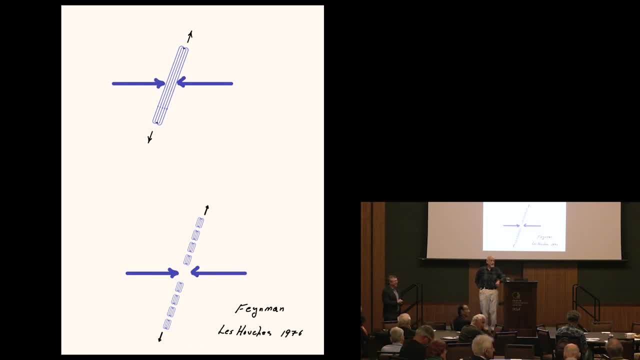 about holography and the boost of repartons that creates this cloud Right Like holes. so I just referred to it, Right? I'm not sure what to say about it. Yes, of course it was an extremely important part. 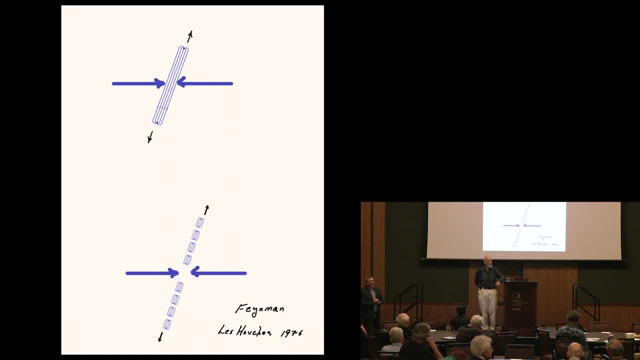 of the whole story: The parton-like behavior of hadrons and deep inelastic. I assume you're talking about deep inelastic electroproduction. Yes, I decided not to try to talk about that just for the sake of time, but it was very important. 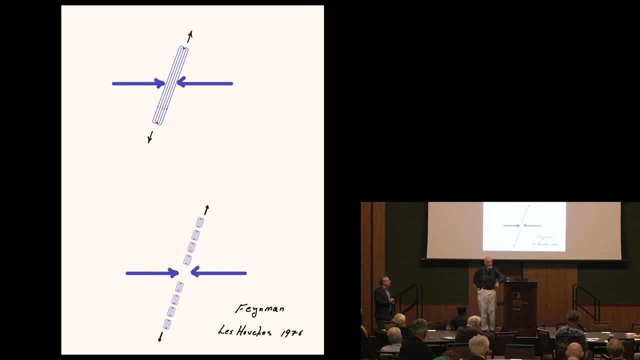 It is, I think, the place and the time when it just became clear: are quarks real or are quarks not real? That's a matter of definition, But I think it became clear at that point that it was useless to take the definition. 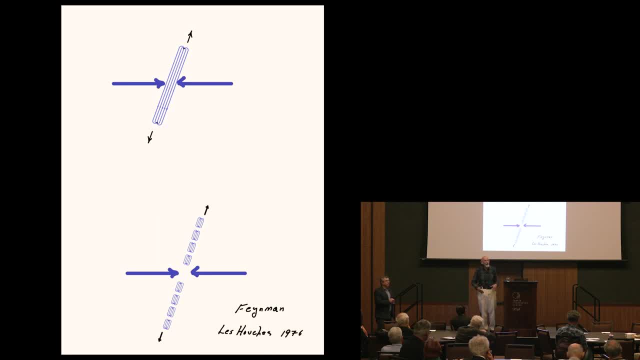 To take the definition where quarks were not real, Everything was pointing to, it would be a stupid definition to say that quarks were not real And that, to my mind, came from two things. It came, of course, from asymptotic freedom. 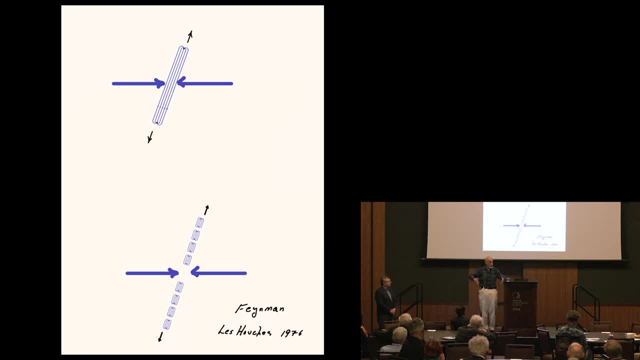 but that was later and earlier from the deep, inelastic electroproduction experiments, And I think that's the way it came to be. But I think that's the way it came to be. Lenny, what is your idea for where the glue balls are? 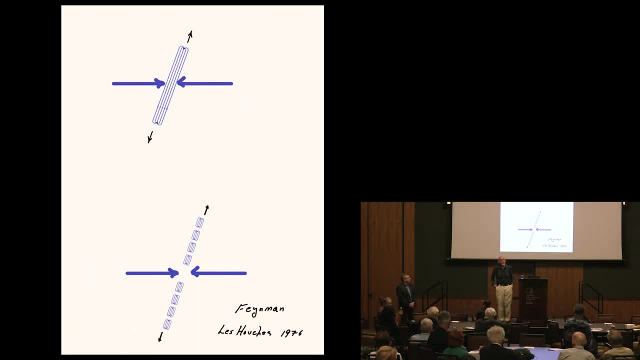 specifically the two glue-on glue balls. Well, as I said, I've been away from QCD for 43 years, So I would have to ask you an exp—. I had a load of difficulty even finding the regit trajectories for these other particles. 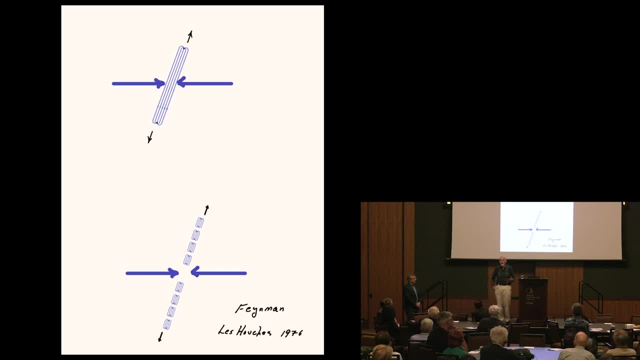 I did find some regit trajectories for glue balls but I could not tell whether it was theoretical or experimental. But from the Okay glue ball, glue balls are closed strings. Because they're closed strings, the two end, the two branches of the closed string, 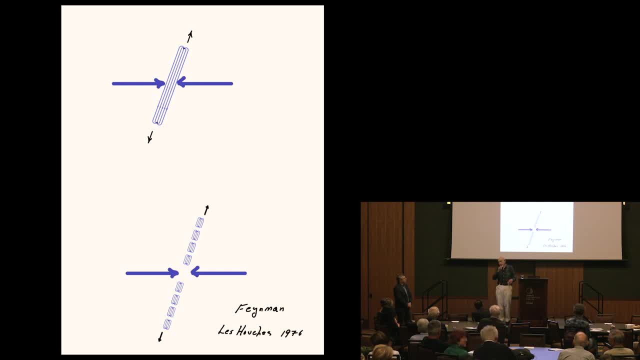 have a lot of opportunity to intersect themselves And I think it's somewhat natural that the glue balls would be distorted. Incidentally, the glue ball trajectories have theoretically half the slope, I think. if I understand correctly, glue balls are, if they have any regi— picture at all. 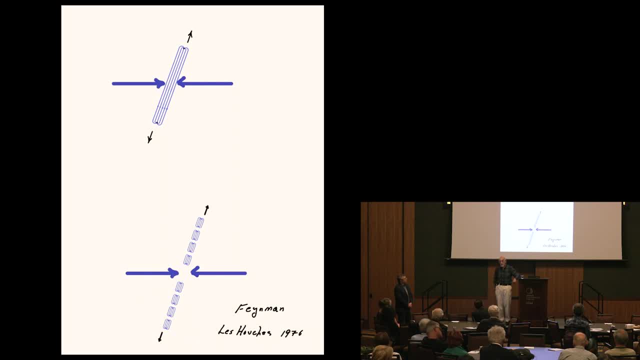 the slope is more like one third of the other particles, But I wouldn't be at all surprised if it was as messed up as the daughters, but I'm not sure Right. Also, Lenny, you didn't mention very much your work on deconfinement.